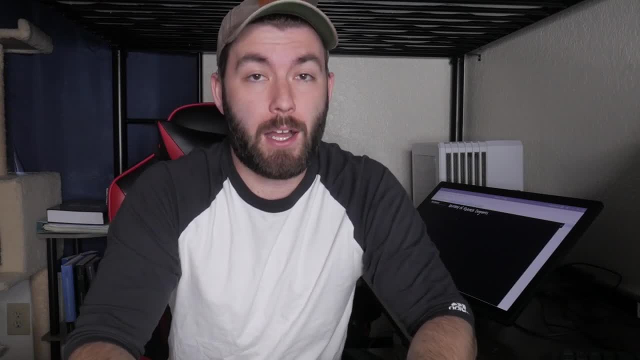 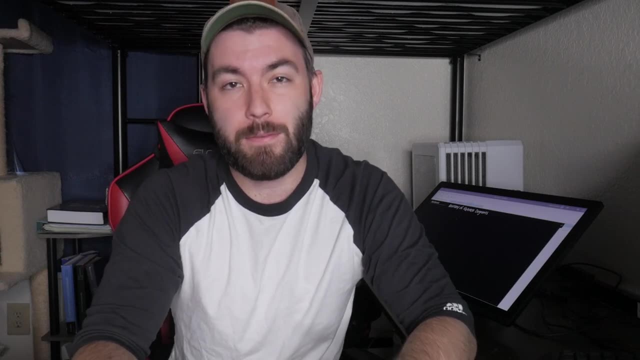 What you may not know is that every Feynman diagram is actually a mnemonic for usually a pretty complicated mathematical expression. Now, this video is not going to show you how to calculate them specifically, but rather we're going to dissect the parts of the Feynman diagram. 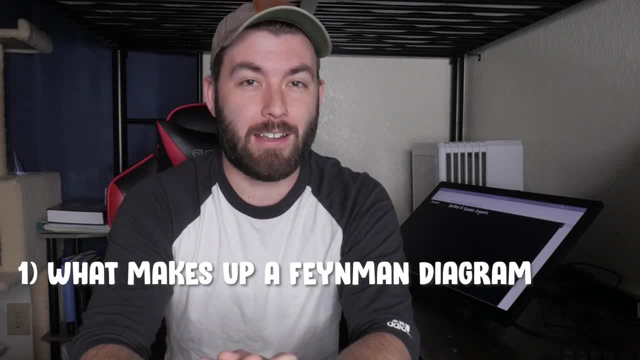 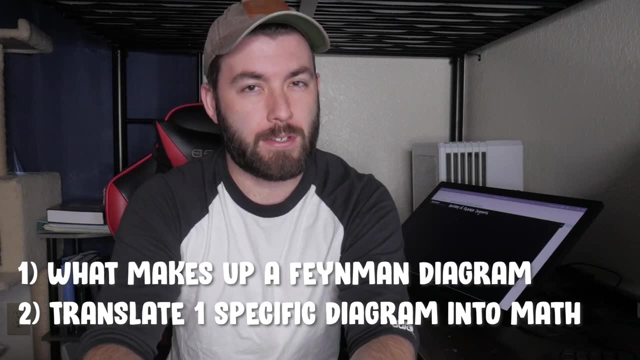 and show what the individual parts are. Then we'll pick on a specific diagram in a particular quantum field theory and show how we can translate it into the math. but we're not actually going to solve it Now. if you've already taken quantum field theory or if you know QFT, you're probably not. 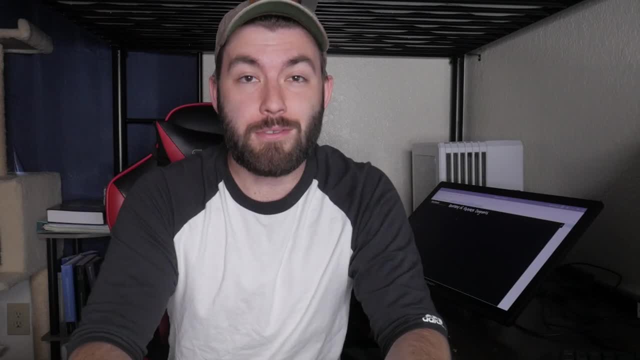 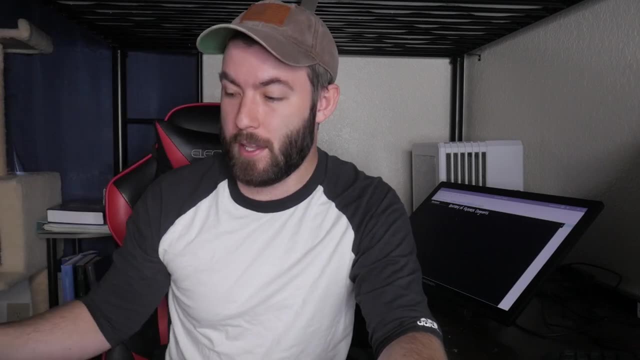 going to get anything out of this video. This is for those of you who are interested in QFT but maybe aren't far enough in your studies yet to really dive in completely into Peskin's Schroeder just yet. Once you understand the anatomy of a Feynman diagram, the rest is just 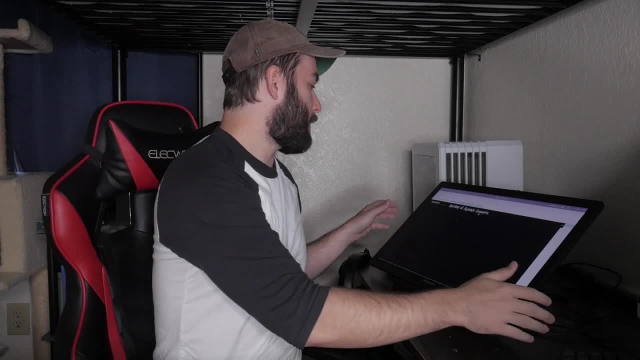 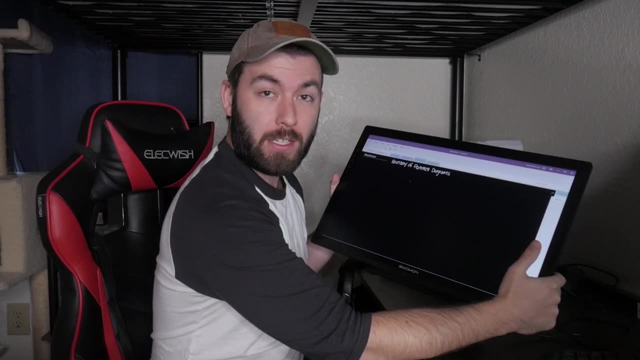 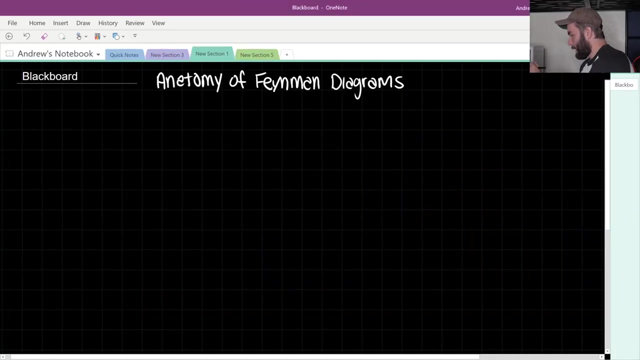 quadrature, as they say. Now I'm going to be doing all of this video on the Gaumont PD2200 that the folks at Gaumont were nice enough to send over to me. If you like what you see and you want to find out more, stay tuned towards the end of the video, where we talk about this a bit more. Now what is? 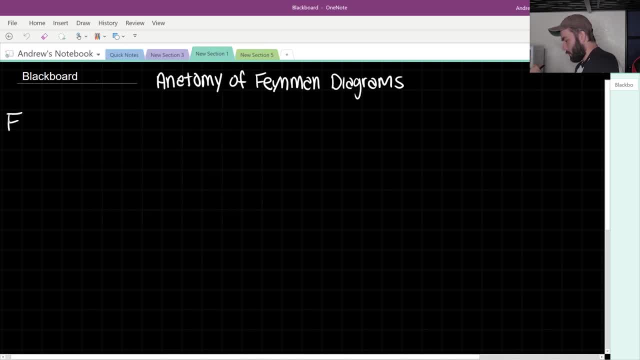 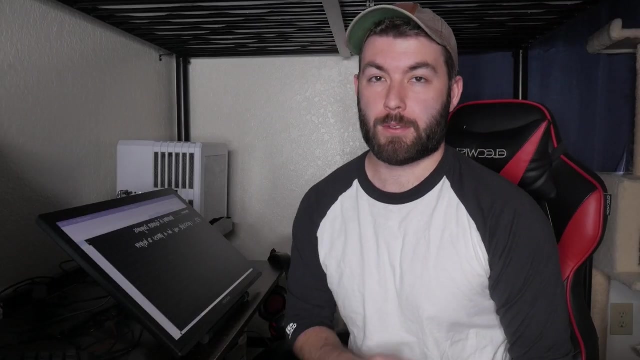 a Feynman diagram, So we said this a bit earlier. a Feynman diagram is one possible way for a process to happen. I'm being pretty careful with how I'm stating this, because there's a very wrong way to say this and a very wrong way to interpret Feynman diagrams, and it's a shame. 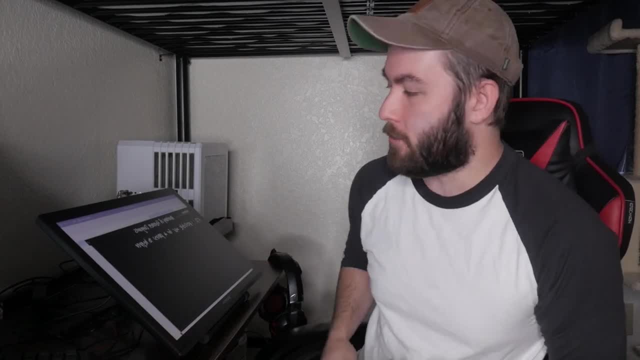 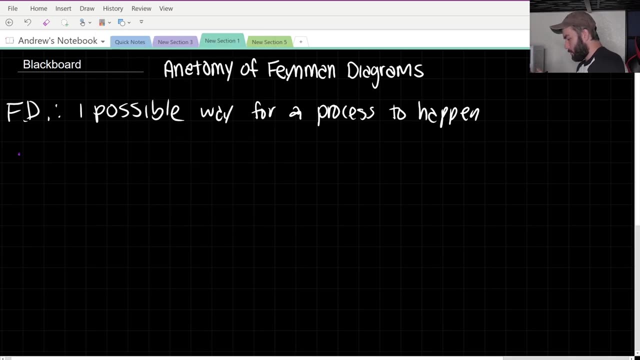 because the wrong interpretation is much more intuitive, as it usually is. Now, what do I mean by process? Well, a process, you know you start with something. you know you start with something. let's say that we have two electrons. one has an initial momentum, P, another one, 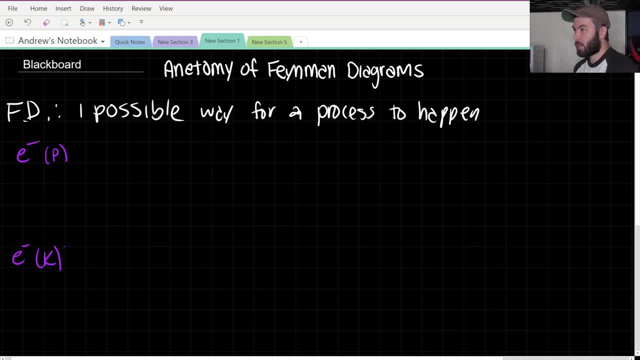 has momentum K, and then we want to measure outgoing electrons. maybe we're looking at the outgoing electrons- they're gonna scatter, or the these electrons are gonna scatter, and then I'll have momentum P prime and K prime. a Feynman diagram would be one possible way of this happening. one possible way. 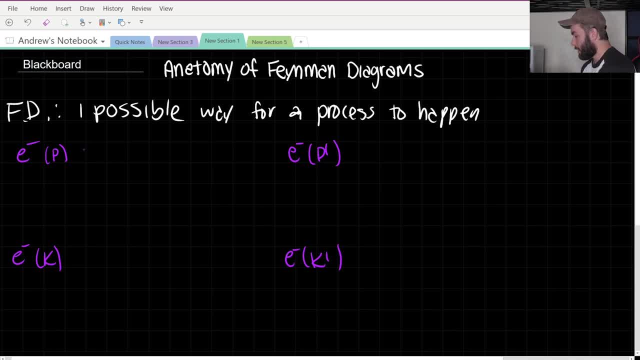 well, if this is an electromagnetic interaction, which is which it is, there should be photons involved when they scatter so around. at this point we would draw the exchange of a virtual photon, which is typically denoted with a gamma. now, conservation of momentum: if, if the first electron starts with momentum P. 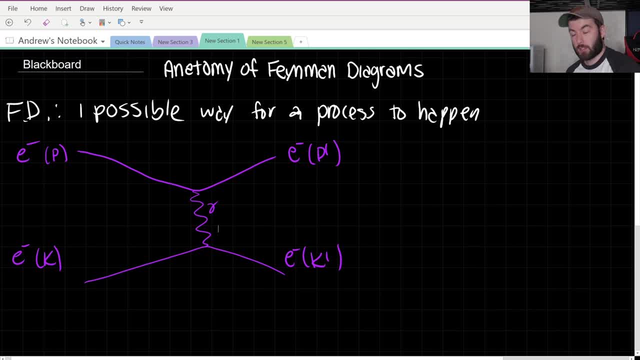 and ends with momentum, P prime. where did that momentum go? well, that momentum is Q, carried by the virtual photon, equal to P minus P prime, because that's one possible way that it happens. the main takeaway, though, or the big thing, that is a huge source of confusion with. 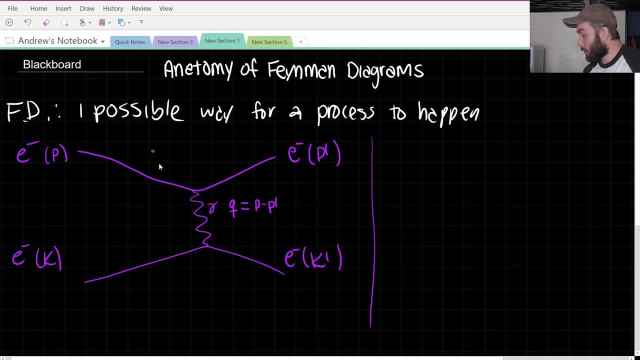 people first learning Feynman diagrams is understanding that you are not measuring what happens in between by definition of where your detectors are. you are measuring these external lines- here you're measuring the electrons leaving and that you also assume that you know the properties of the, of the 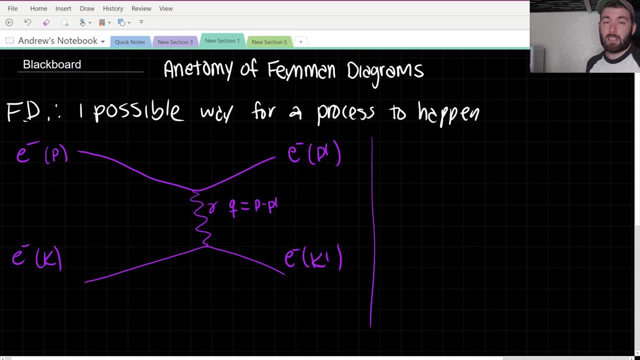 electrons going in your detectors. not being there means that you can't tell if this is what happened. or maybe this is what happened: the electrons scatter, but it's a bit more complicated. maybe that virtual photon split into a particle antiparticle pair which recombined into the same, into a photon. 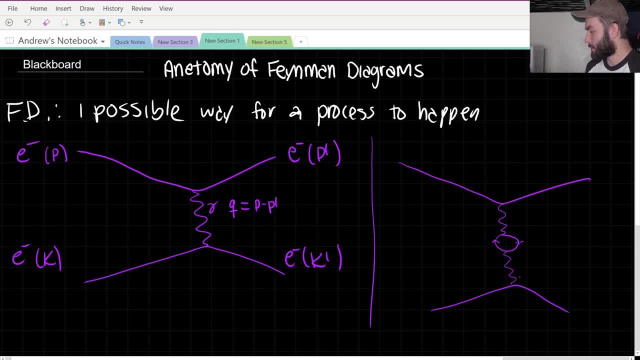 and then you get a process like this right. so the Feynman diagram is a possible way for something to happen. in order to calculate the total probability that something happens, you have to add them all up. you have to account for everything. however, you're not specifically claiming that any one Feynman diagram is. 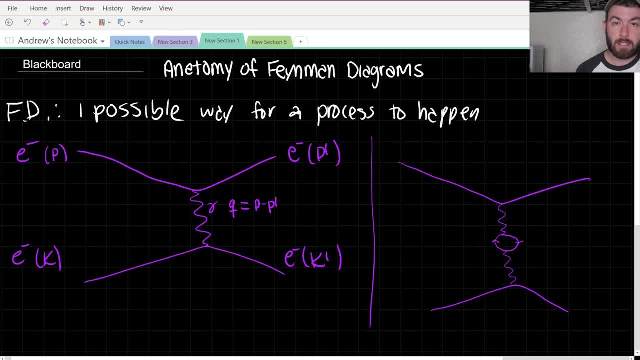 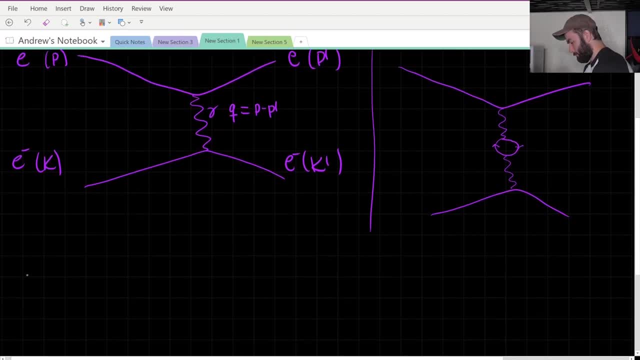 what happened because you're not measuring the intermediate stages. that's very important. so, formally, what a Feynman diagram is formally, and I'll describe it formally once and then we'll move on, because I understand people are at different stages. all a Feynman diagram is is a term in. 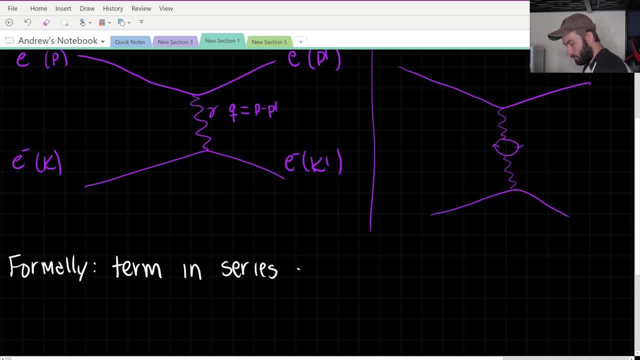 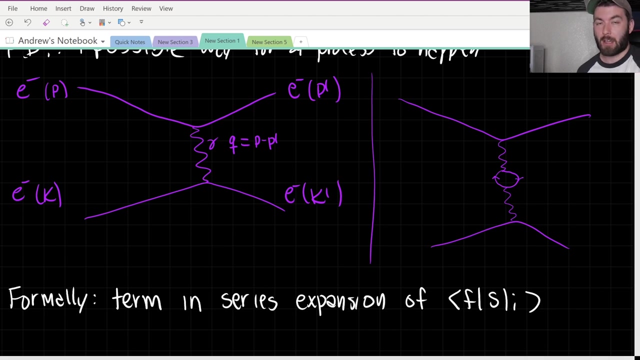 a series expansion of something called the S matrix. so it's a, it's a term in a perturbative series. if you've done perturbation theory before and just like in perturbation theory, eventually you say let's not go to infinite order, that's going to give me contributions that are not worth the effort to. 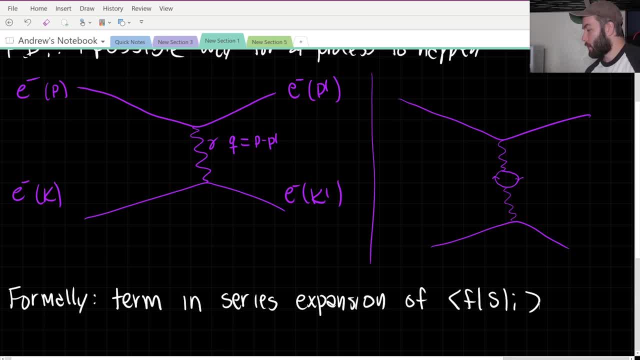 calculate. so let's stop at a certain order, and in which case maybe this one is in the orders that I'm not considering anymore, in which case I only get the simple guy, and then I'm tempted to say that that's what's happening, that's what I'm measuring, but in reality you cannot make. 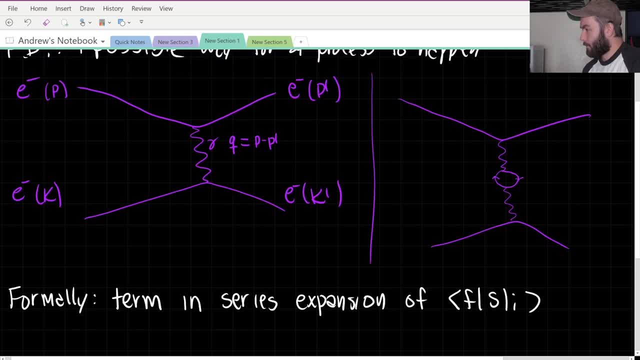 such claims okay. so this is kind of like if you were going home from work and if you're going home from work and I have to calculate all the possible ways that you could go home, one of those possible ways is you taking a pit stop around the. 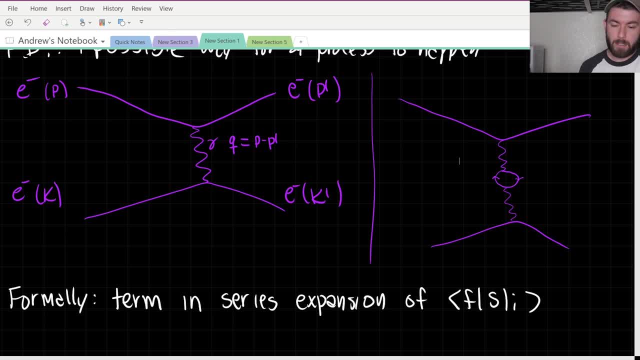 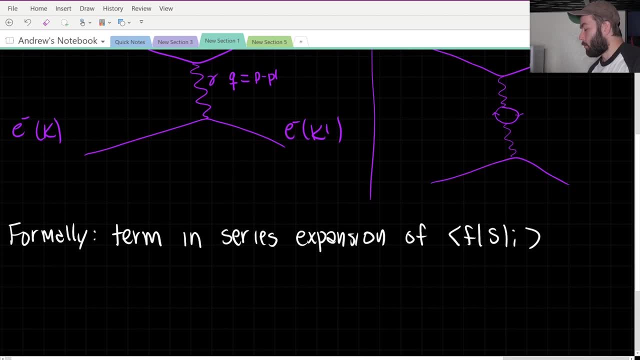 world right. but that's not very likely and it probably doesn't add much to the accuracy of my calculation if I neglect that contribution. so in principle, if I want to calculate a cross-section I have to add up all of the diagrams. for specific reasons it's squared and in general there's going to be infinitely. 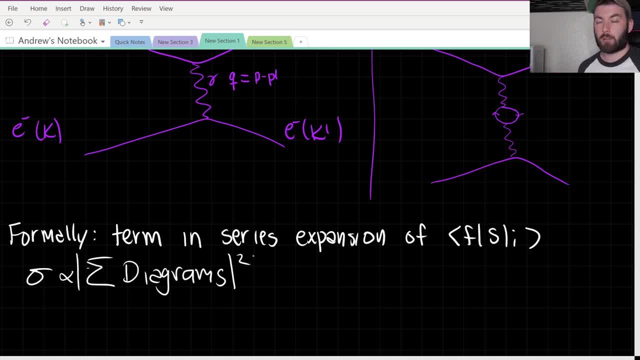 many diagrams. so we're very lucky that as a general rule, the more complicated the diagram is- and in a bit I'll explain what I mean by more complicated- the more complicated the diagram is, the less it will contribute to the total probability. so we end up truncating that series at a certain point and neglecting what are. 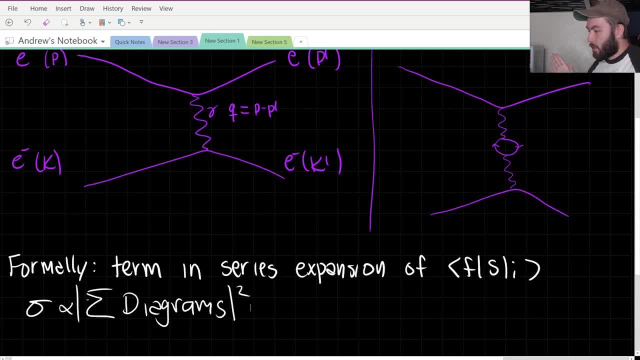 called the higher-order contributions. so, at the end of the day, you don't measure a particular Feynman diagram, you measure adding up all of the diagrams, which may sound weird if you're you're not sure what you're talking about. we're adding together a bunch of pictures. what does that mean? well, these. 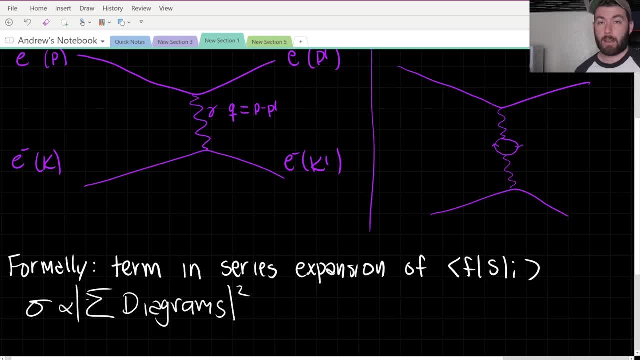 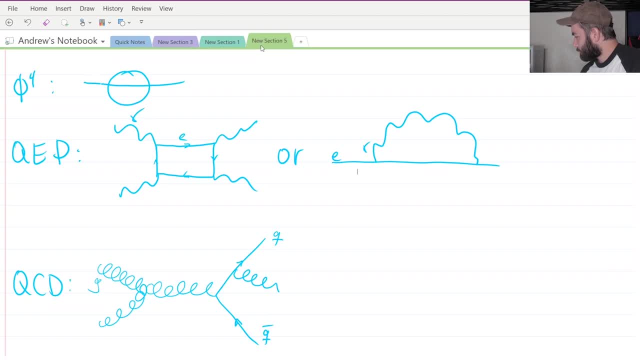 Feynman diagrams stand for literal mathematical equations and what they stand for depends on the quantum field theory. so if we go over to this tab, I've written down a couple. this is far from all the diagrams you could have, but I've drawn a couple examples of diagrams in various quantum field theories. so this: 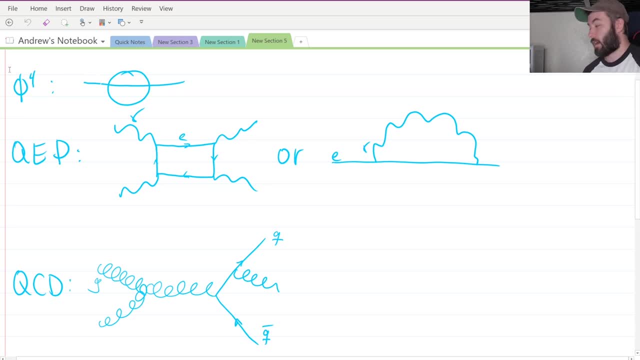 is the one of the more simple quantum field theories. it's called five four. it's a scalar field theory and this is one of many diagrams that is allowed in quantum electrodynamics. we have multiple kinds of particles, we have electrons and we have photons, so those should be depicted in a different way diagrammatically. the 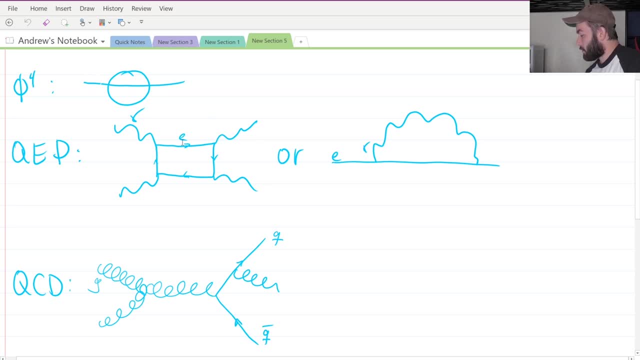 wavy lines are photons. the straight lines with the direction with these little arrows are electrons or anti electrons, positrons. this is one interesting little diagram. I find it interesting because you're normally taught that photons can't interact with each other, and what that comes out to in Feynman diagrams is: you never see photons. 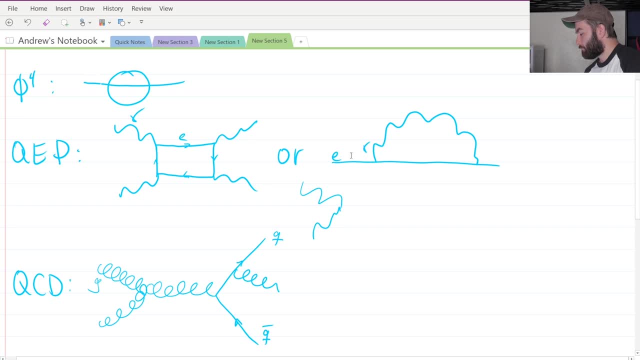 directly connected in a diagram. however, this is one of those loopholes where they can actually interact. it would just be an example of them only being able to interact at higher order and perturbation theory, which is kind of cool. another example is a very important diagram that's known as the self-energy. 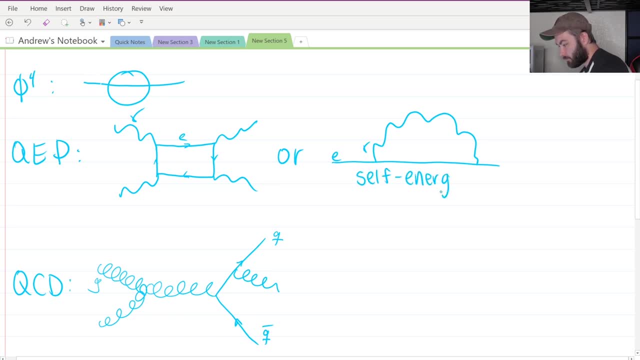 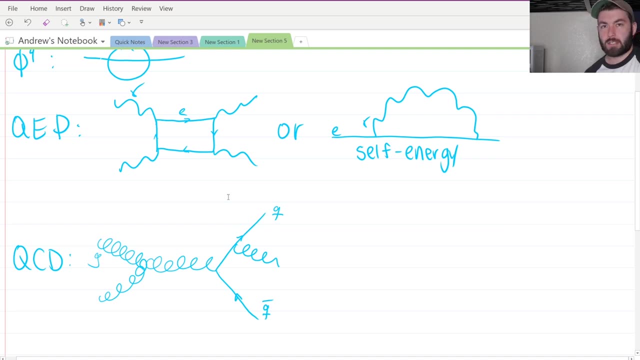 very important diagram in quantum theory, quantum field theory and then in quantum chromodynamics. we can have a lot more interesting diagrams, in my opinion, because the theory just allows for it, on how the particles are allowed to interact. we can have these bosons, in this case gluons, meeting up together, and then we have these external lines that 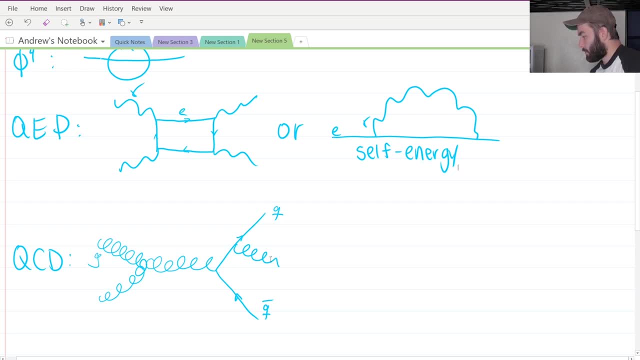 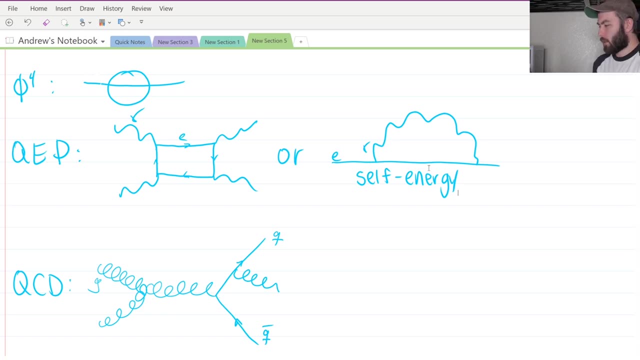 are now quarks and gluons, this radiative correction here, but the point is, we have all of these different diagrams for different kinds of quantum field theories. the question that we then ask ourselves is: hey self, here's our little self. what do these have in common? 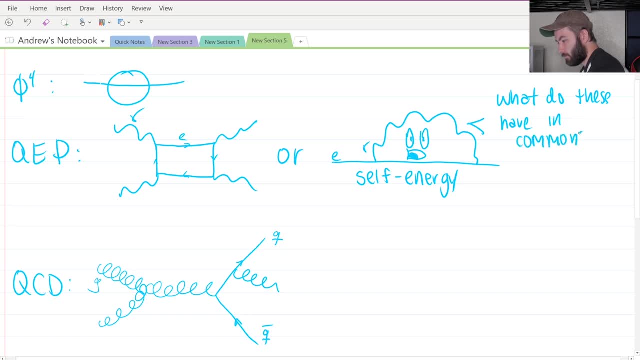 have in common? they all look very different, but they do have properties that are mutual among all of them. for one, we all have incoming and outgoing particles, and those are denoted by these external or the these external lines. these internal lines are the incoming particles. sorry, these external lines, here coming in, are the. 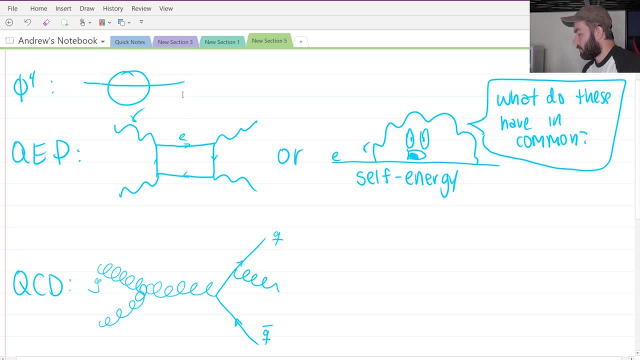 incoming particle and this external line leading out is the outgoing particle, and the same goes here. it's just what is that particle? now, since we'll talk about this in a bit, since these are different particles, they should probably stand for something different mathematically, which is something that 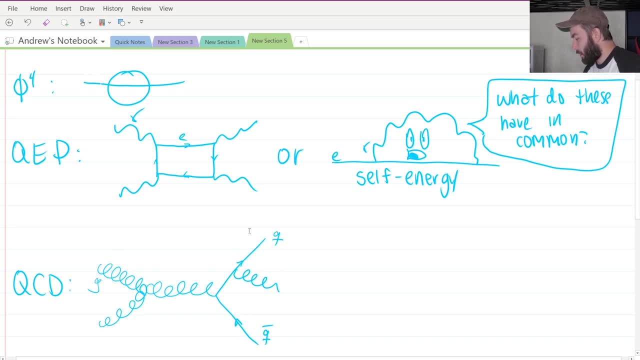 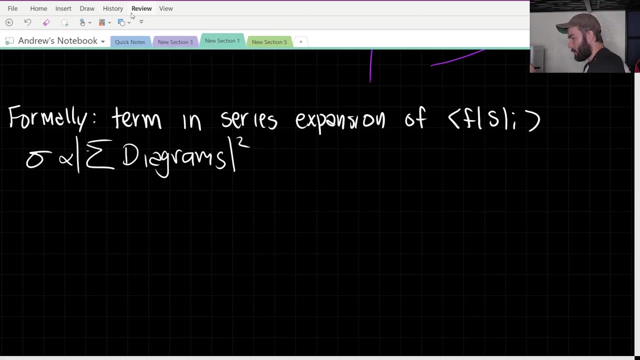 we'll get into. but that doesn't change the fact that in amongst all the Feynman diagrams we have external legs, these external legs that aren't leading necessarily to anywhere else aside from our detector. so if we start creating our are documenting our dictionary or not our dictionary, our components of the 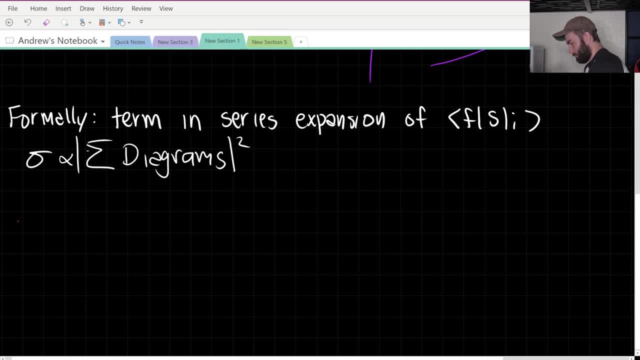 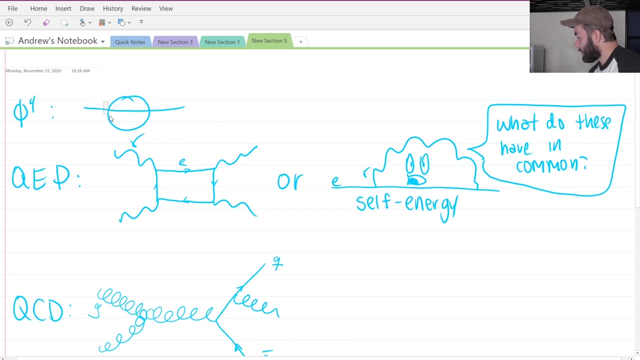 diagram. let's do it in people- the anatomy. our first entry is going to be external legs- sorry, if you can hear- my computer can't really do anything about that now- where these external legs going or coming from these external legs are either going to a vertex or coming from a vertex, so in scale or field theory. 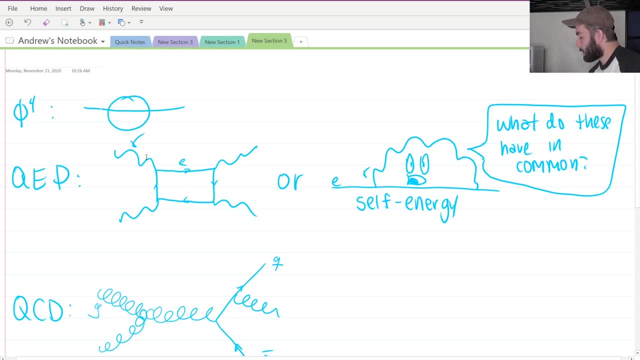 that's the case in qed. we have three lines coming or going. so we have one line going to a vertex, then a vertical line and then a vertical line and then going to each other- and we'll talk about this in a minute- two leaving and so on, or two, depending on how you read it. so in QED you have three vertex with three. 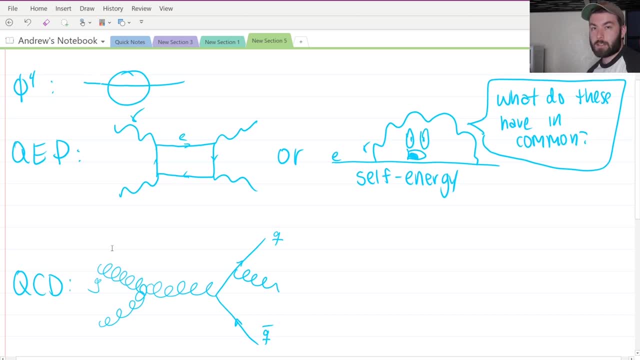 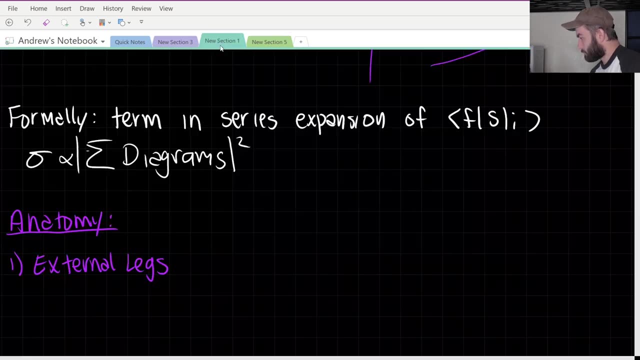 lines. and then in QCD- I haven't drawn the diagram here, but you can have three or four, but at the end of the day you still have vertices- you have these lines going towards vertices, okay, so that's going to be our next part of the anatomy. two vertices, okay. is there anything else? well, yeah, there. 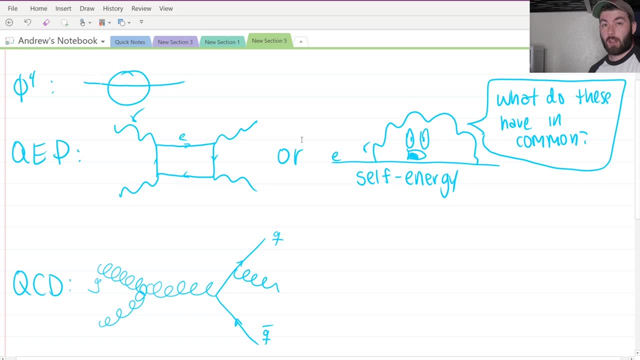 actually is. if we have two vertices, then we may have lines connecting them. so here we have a vertex here, and we have a vertex here, and then we have a line. here we have three lines connecting them. whenever you have a line in between vertices or connecting them, that's called a propagator. 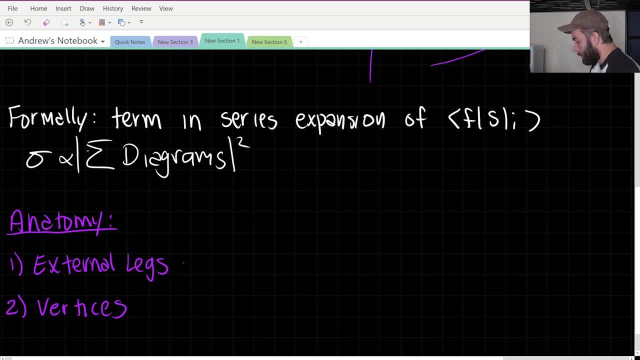 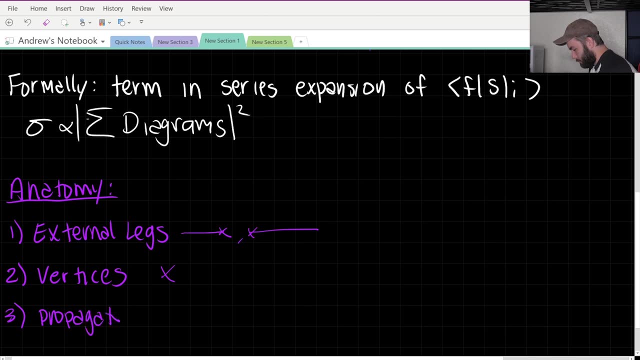 those internal lines are called propagators. so let me draw this stuff for us. we have lines either coming or going to vertices of our vertex, three propagators. I have no idea if I'm spelling this stuff right. by the way, propagators are would be lines in between vertices. okay, regardless of the quantum field theory, these are the three parts. 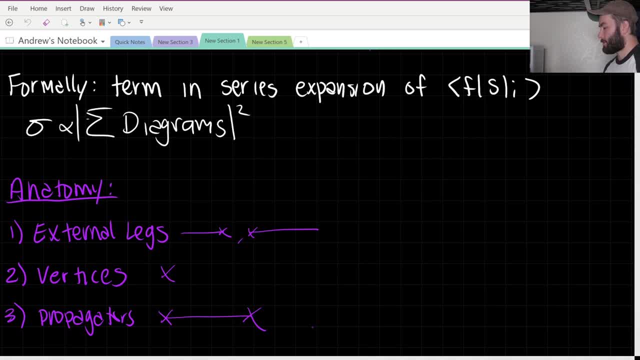 that make them up: vertices, propagators and external legs. the big thing, the only difference now, is how we are allowed to combine these. how can we combine these lines and vertices? how to combine- or how we can combine, i should say it can combine- depends lips on that qft, on the quantum field theory specifically. 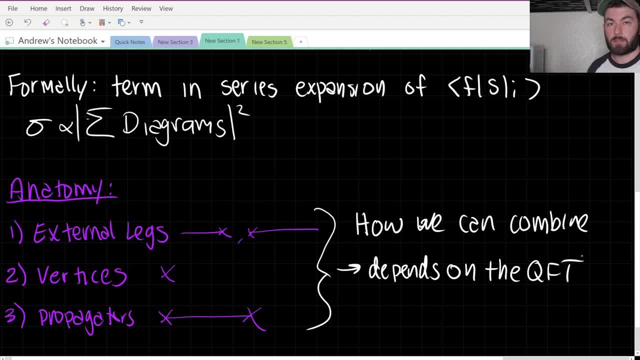 on that qft on the quantum field theory, specifically on that qft on the quantum field theory. specifically, it depends on the Lagrangian right, it depends on the equations of motion. how are these things allowed to interact? that determines how we are allowed to attach these lines and propagators. okay, so let's do a little example. so for a 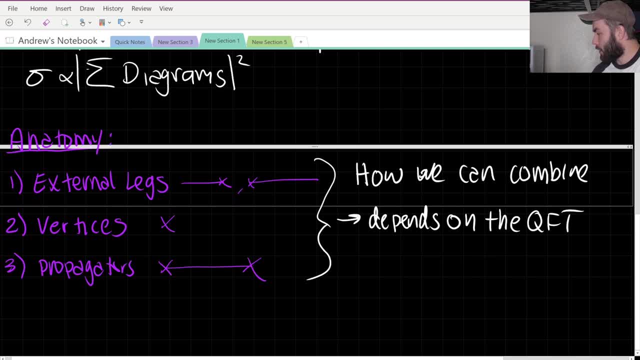 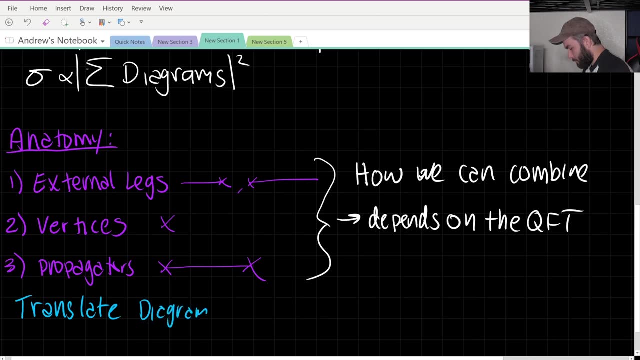 particular quantum field theory. how one translates the diagram into the math is determined by what's referred to as the Feynman rules. so translate the diagram into math. you use the Feynman rules. he sure does. and there will be Feynman rules for every quantum field theory, and there should be, because these particles 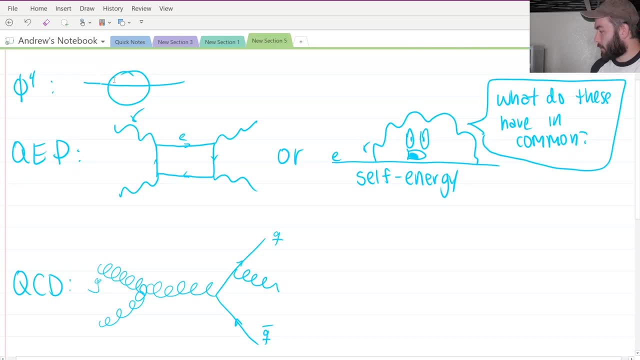 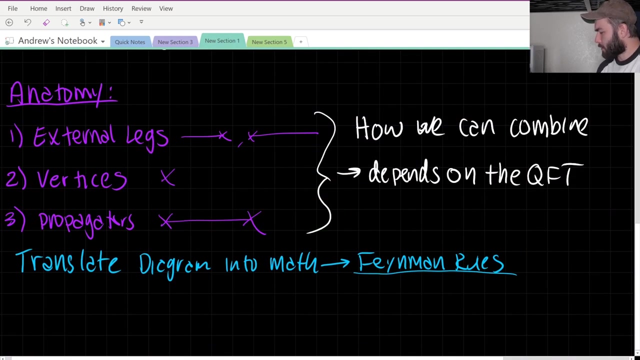 interact in different ways. how a scalar field interacts, how scalar fields interact, is different from how a gluon interacts with a quark. so how we translate the diagram into the math should it should- depend on the theory. okay, so let's go ahead and pick on a particular theory in a particular 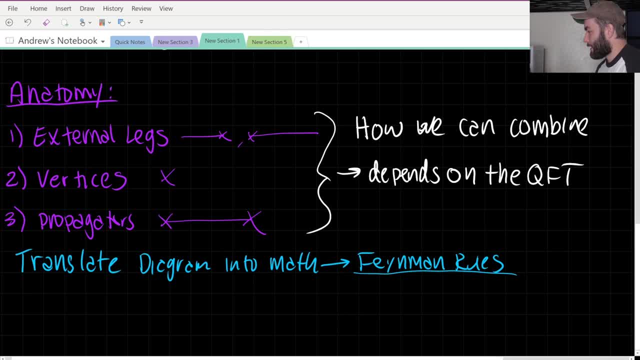 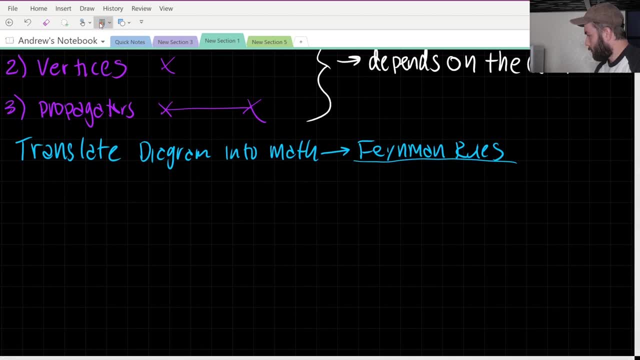 diagram within that theory and see how we can translate that, given Feynman rules which I'm just going to give you. so let's do, let's do a scalar field theory. so let's do Phi, let's do Phi cubed, which is another scalar field theory, and for the scalar fields, it. 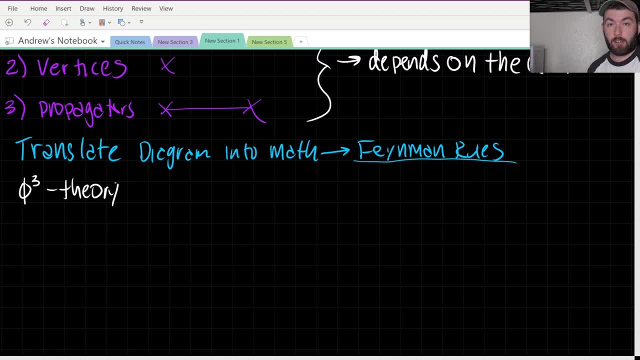 doesn't matter if it's it, how you're allowed to attach them. the diagrams that pop out depend on the theory, but the Feynman rules. what the legs and stuff stand for is the same for the scalar fields, so the first of which? let's go ahead and let's let's draw a diagram one. 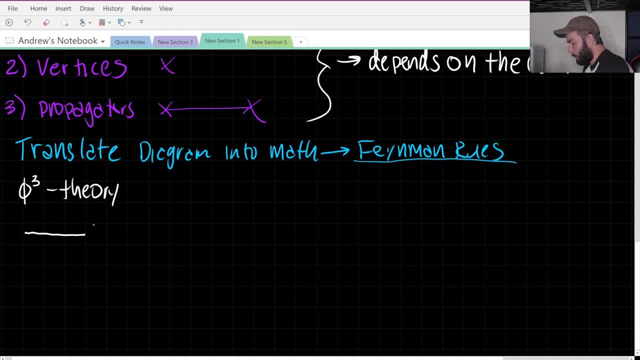 possible diagram, let's do. let's do this. the equivalent of the self-energy for Phi cubed. so if it's three, that means that there will be three lines at attached to the vertices. Phi to the four means that there would be four lines. so let's make. 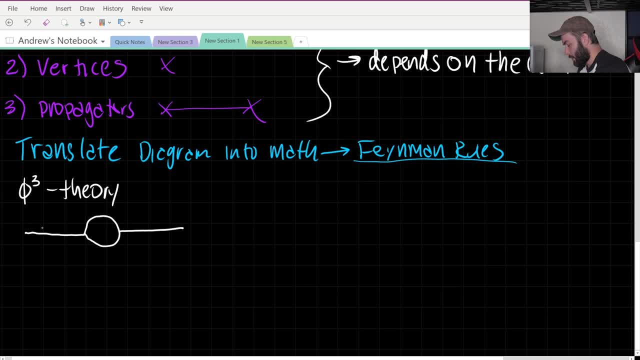 sure that we only have three lines, and let's denote this as P, P, prime. we'll call this k1 and we'll call this k2. why not? ok, let's go ahead and draw lines, just for good measure. ok, now, how do these rules translate for a specific field theory? so for one. 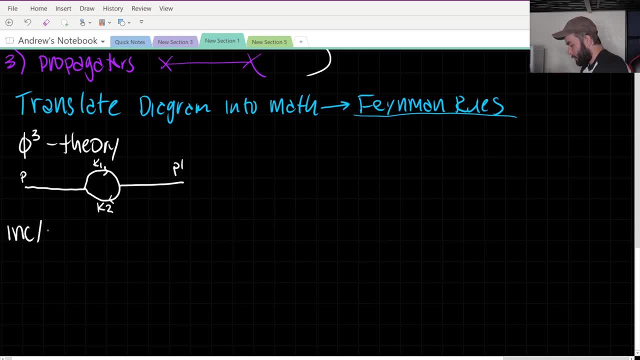 external lines- i'm gonna write it is incoming outgoing lines are given by an exponential e to the minus plus P dot X. where X is is like this point of where the vertex is, P is going to be the momentum associated with that line. in the external line we have a P prime, so we would call it P prime and 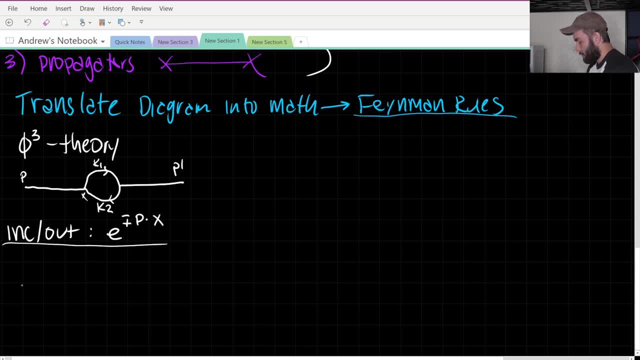 so on. okay, so that's one. now for the vertex. that's where the interaction happens, and interactions depend on the coupling strength, depend on the strength of the interaction. so in a scalar field theory, the every time we see a vertex we multiply by minus, I times the coupling constant and then 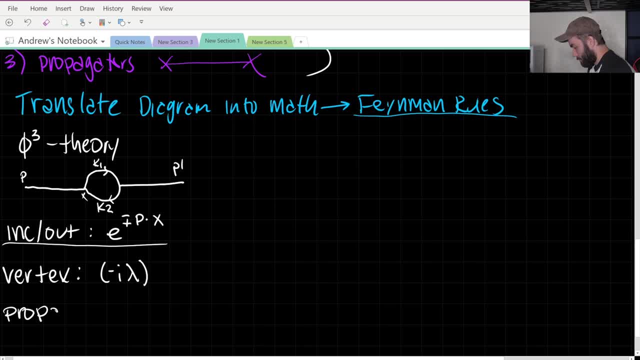 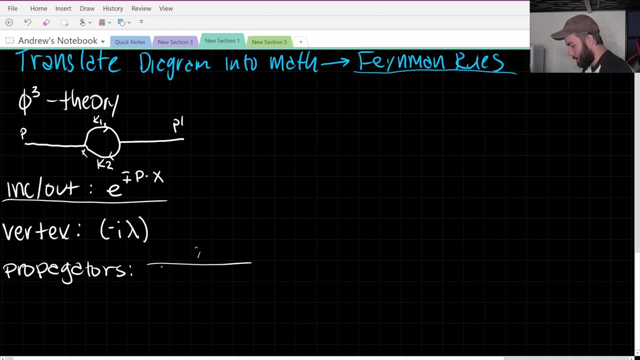 lastly, we have our propagators. this is given by solving for the equations of motion for the particle and for the vector of motion, for the vector of motion, for the vector of motion for a scalar field. it is given by an I divided by. I'm going to call it K K. 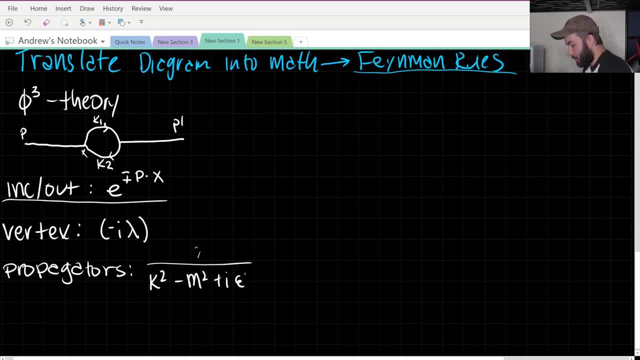 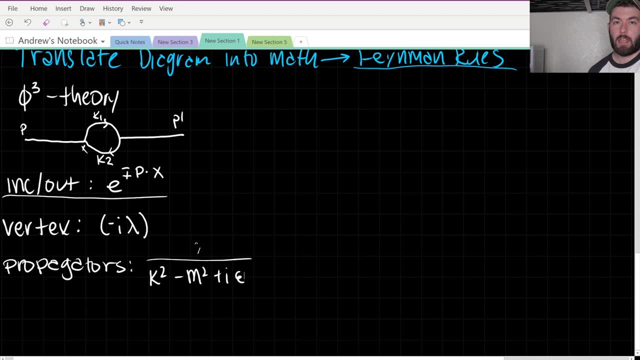 squared minus M, squared plus I- epsilon. and then there's going to be a few more caveats to this that we have to make sure that we're imposing. one momentum should be conserved, so let me write a little. they're typically lumped in with the Feynman rules, but I'm going to write them as if they're caveats, just because. 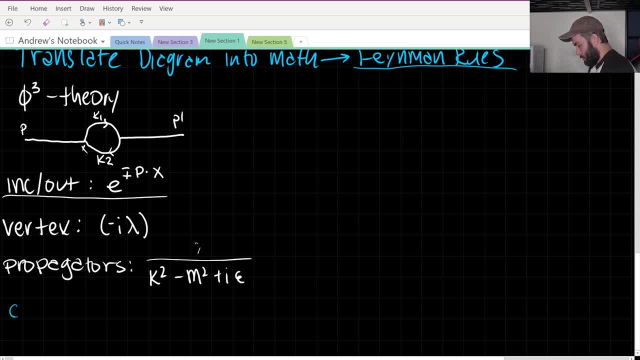 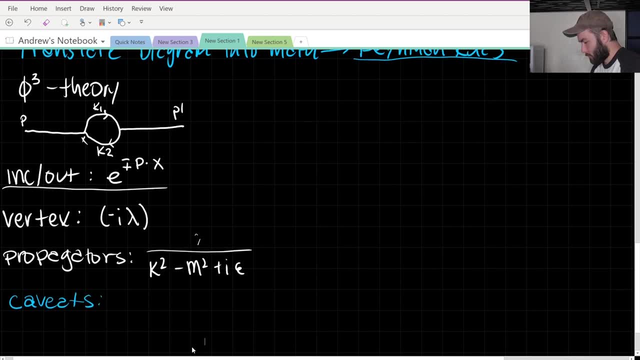 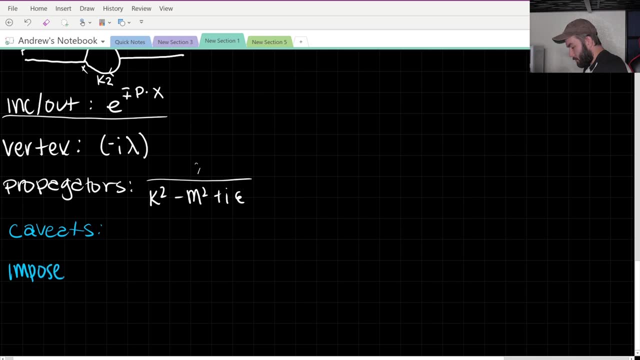 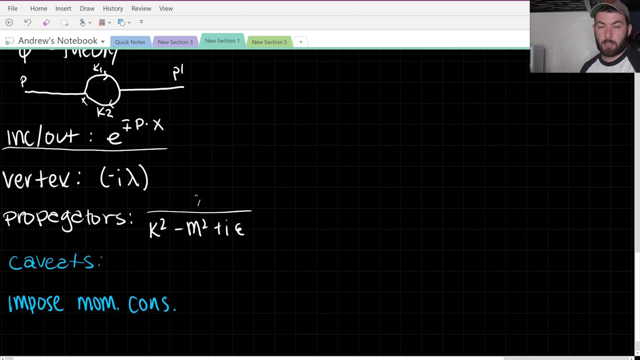 it's not a specific equation that we're giving. caveat is that momentum should be conserved, so impose momentum conservation at the vertices. so wherever these lines are flowing into or coming from should be equal to the momentum that's leaving. we should impose momentum conservation at the. 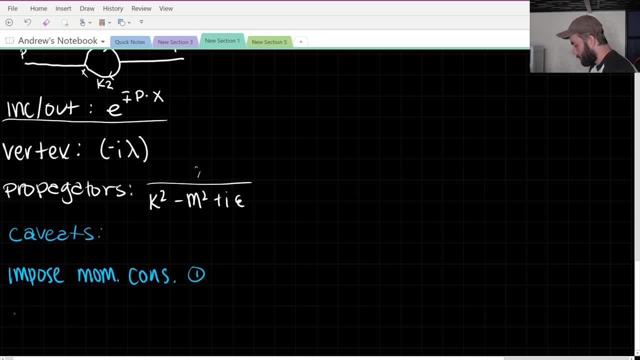 vertices. So that's one And two. we have to integrate over undetermined momentum, So that would be of the form like integral d4k over 2 pi to the fourth. So whenever we have to integrate over an undetermined momentum or whenever there is an undetermined momentum, 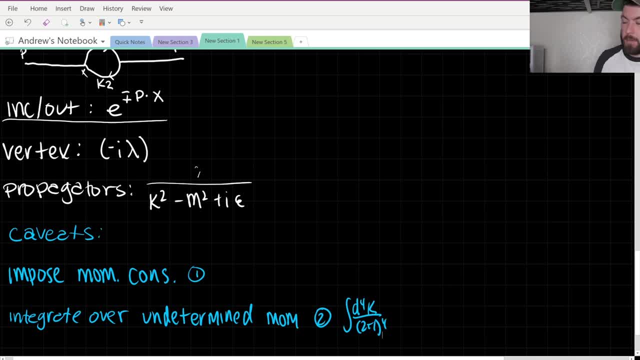 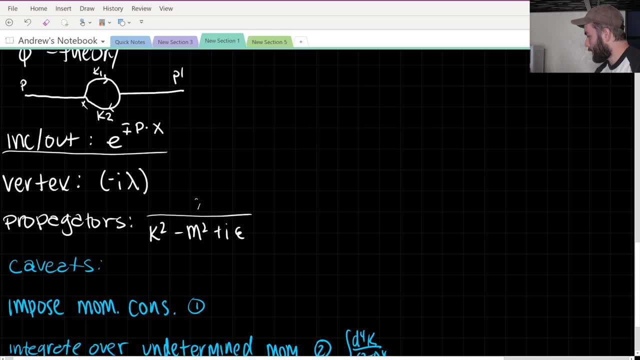 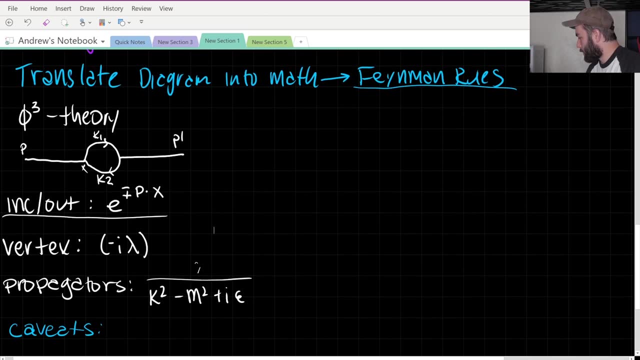 we integrate over the possible values it could have and you weight it by this 2 pi to the fourth. Okay so, with these rules, let's see if we can translate this self-energy diagram into math. Okay so, first things first. momentum conservation tells us that k2 is going to. 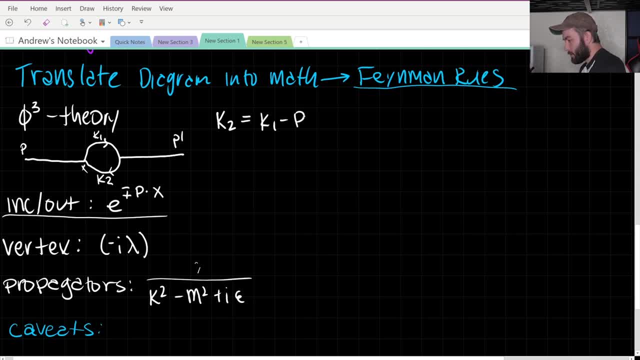 be equal to k1 minus p prime For self-energy. in reality, we should let p equal p prime, but just keeping it general here. that's the case, But momentum conservation at the vertex would mean that k2 has to equal k1 minus p prime. right, Because these are flowing in. 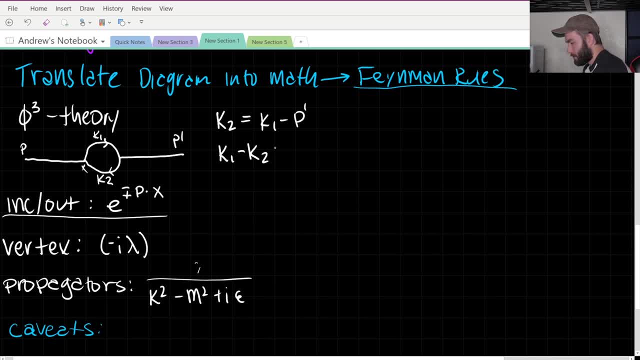 different directions. so we have k1 minus k2 is equal to p prime. So if you solve for k2, that's what you would get. So let's go ahead, So that constraints we don't have to integrate over k2 because we have constrained it in terms of k1.. However, 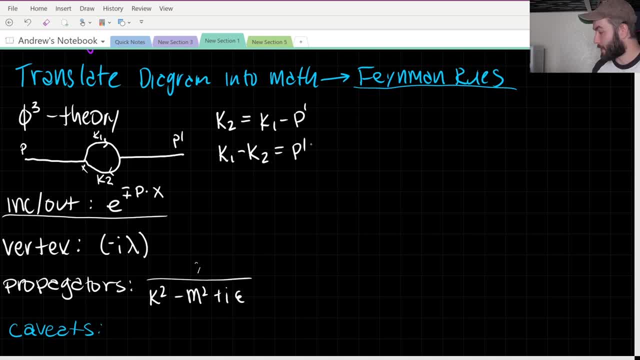 now we don't know. k1 can be anything, because as long as that constraint here is satisfied, k1 can be whatever, from zero to infinity. So that's why we integrate over the undetermined momentum. So I'm going to rename, since there's only one k now. 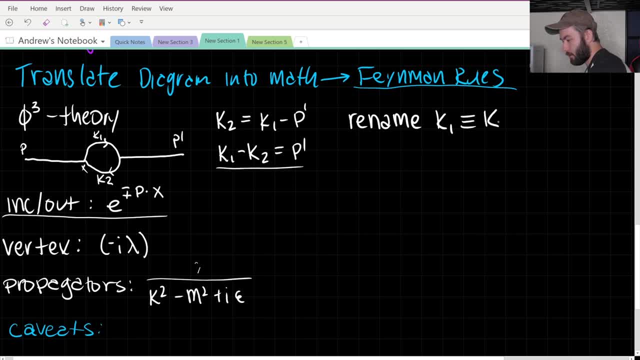 k1.. To just k And let's start writing stuff down. So we see two vertices, We see one here and one here, So that's going to give us a minus i. So this is equal to minus i, lambda squared. Let's go ahead and integrate over our undetermined momentum d4k, over 2 pi, to the 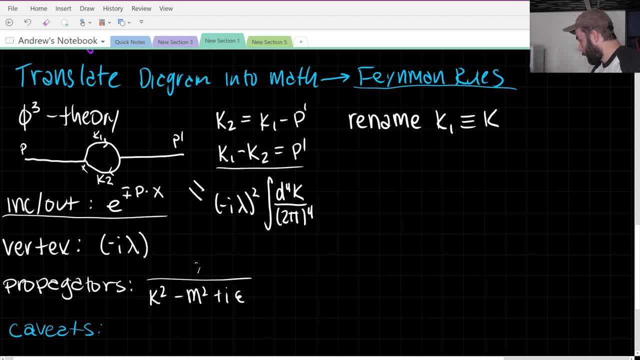 fourth: Okay, now we have our external leg incoming. It's the minus sign. So we get an e to the minus i, p dot x. Then we have our two propagators right here And then we have another propagator here. So when we have two leading to the same point, we get many loop brother. So we have 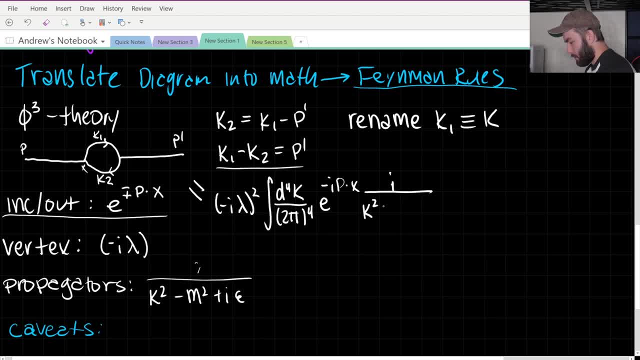 an i over k squared minus m squared plus i- epsilon. That's the top propagator And then the bottom one. well, now we also are just going to substitute, in that k2 equals k1 minus p, i k minus p squared minus m squared plus i- epsilon. 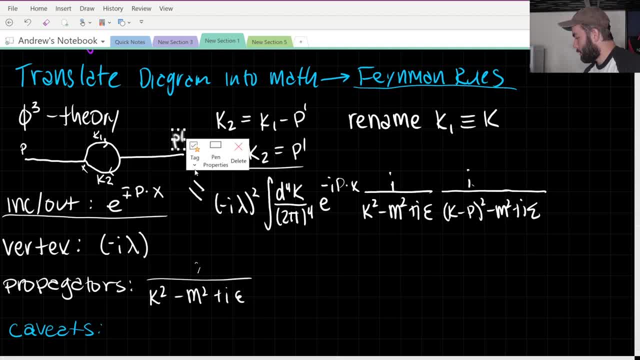 And then, lastly, we have our final external line here, which is given by an e to the i p prime dot y. Let's call this y. That's it, That's the translation. This is our. what we would have to calculate is this integral. 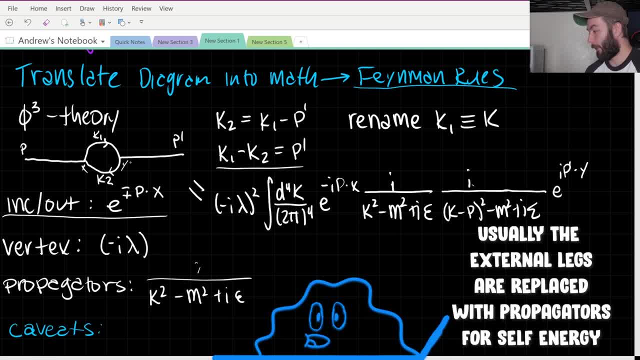 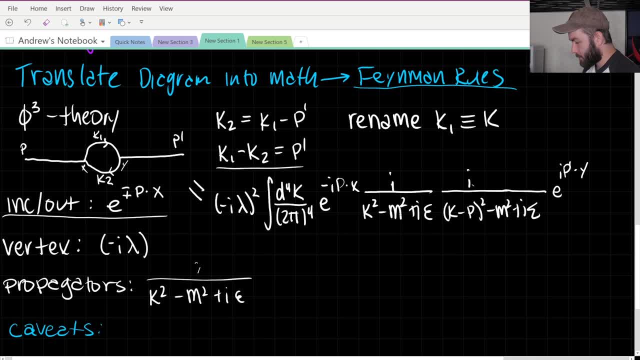 to find the self-energy in the phi cubed theory. The reason we are definitely not doing that in this video is because it's very difficult. If we look at it in terms of powers of k, we see that there are four powers of k. We're multiplying these, So four powers of k in the 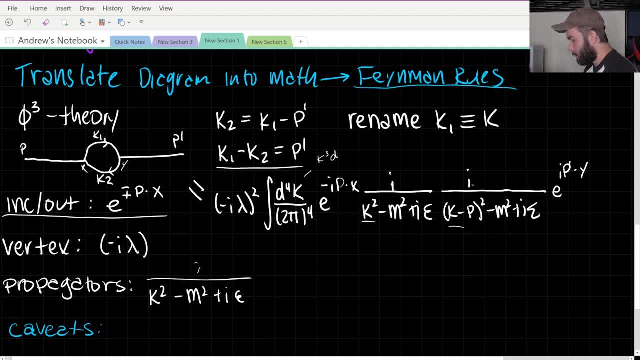 denominator and something that looks like a k cubed dk in the numerator. So what we'd end up integrating goes as k cubed over k4, which, for large values of the momentum, goes as one over k, which goes as ln of k. So we get what's referred to as a logarithmic divergence. 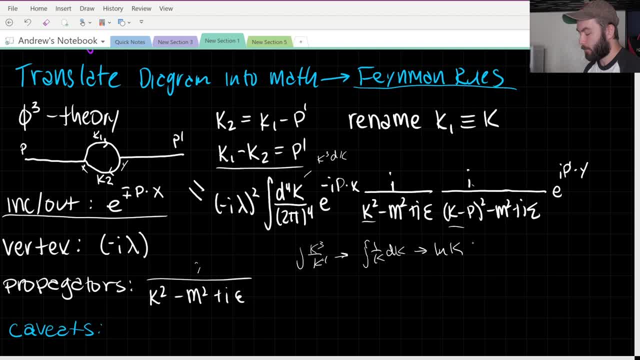 This integral is infinite, is formally infinite, And we'd have to systematically remove it through the process of regularization and renormalization, which I don't think I can do in five minutes, So we're going to skip that. I just wanted to show you one example of how to translate a Feynman. 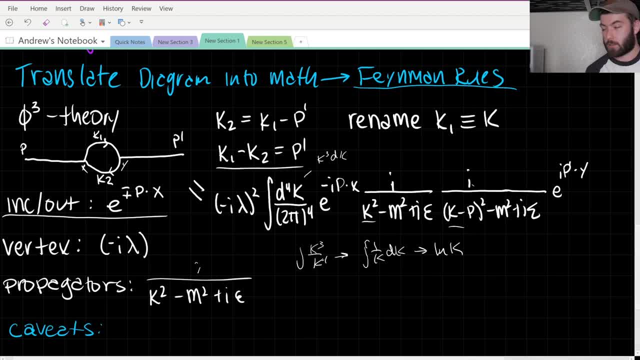 diagram and a particular quantum field theory into the math that we associate it with In quantum chromodynamics or quantum electrodynamics. all you'd have to do if you're given a particular Feynman diagram is really just go into Peskin and Schroeder and look up the 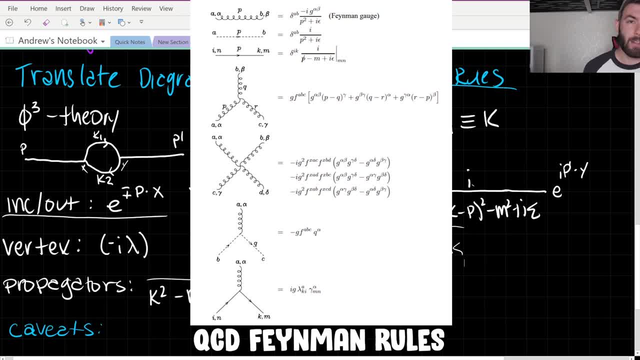 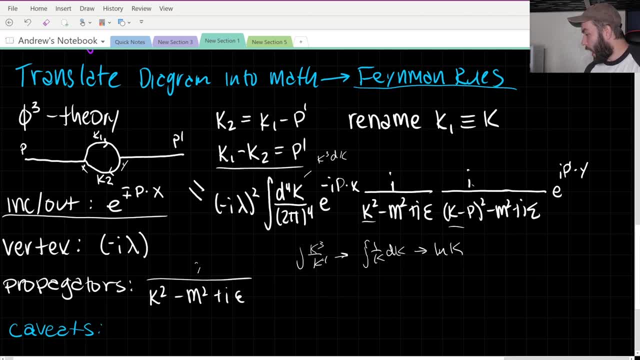 associated Feynman rules, because I wouldn't want to reinvent the wheel for that. You should have to derive them once for yourself. but in actual calculation no one has this idea, So we're going to just go ahead and look at the Feynman rules. I actually wanted to do something on this kind of 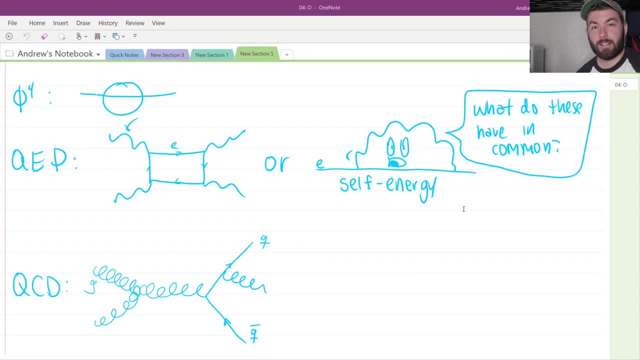 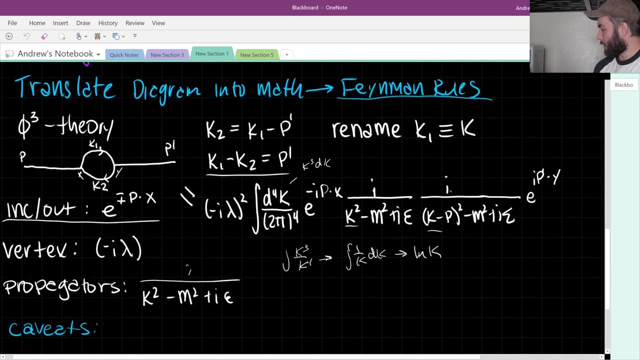 stuff because I didn't even have the time to do this stuff memorized. I looked up the Feynman rules before I made this video. I didn't have the expression for the propagator off the top of my head. One thing that I neglected to mention was what did I mean by saying the more complicated? 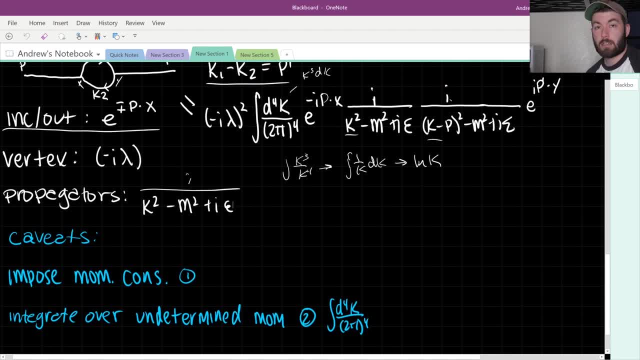 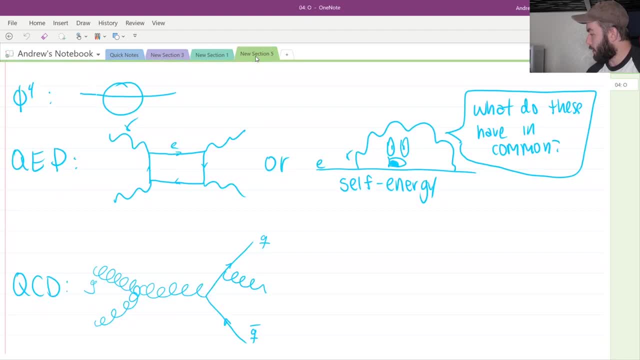 diagrams become contribute less to the total probability. Well, as we saw, each vertex was, it would be the square root of the fine structure, constant. so when we are adding these diagrams to, when we're adding them up to get a total probability amplitude, well, we're multiplying factors of maybe 1 over 137 for every two vertices that. 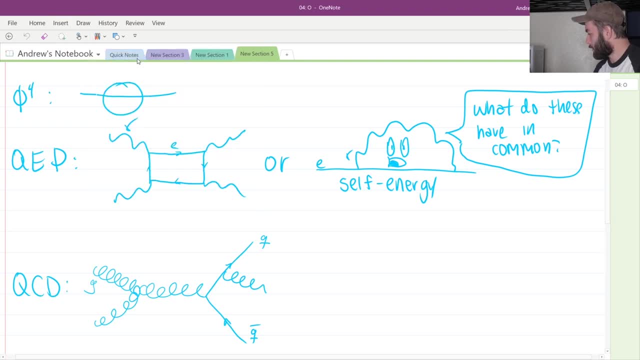 we see, since it's root alpha. so for here you can think of there being a root alpha at this vertex, at this one, this one and this one. so what we're ending up multiplying our diagram by is 1 over 137 squared. so when we're adding this to, 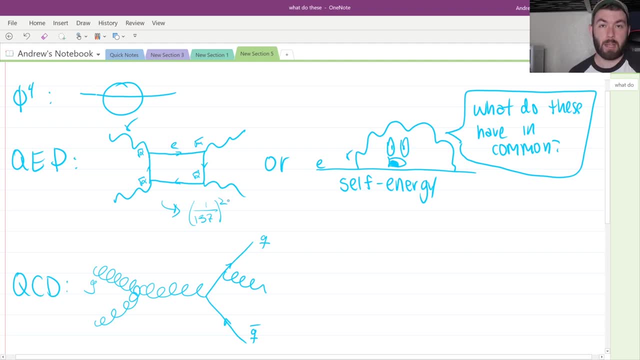 our previous answer. you know it's going to be suppressed by factors of the coupling constant. so that's why these more complicated diagrams- complicated meaning having more vertices- in my eyes they will generally contribute less to the total amplitude, unless there are other reasons why simpler processes are. 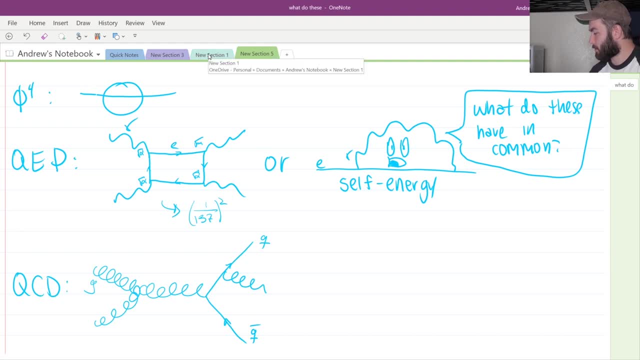 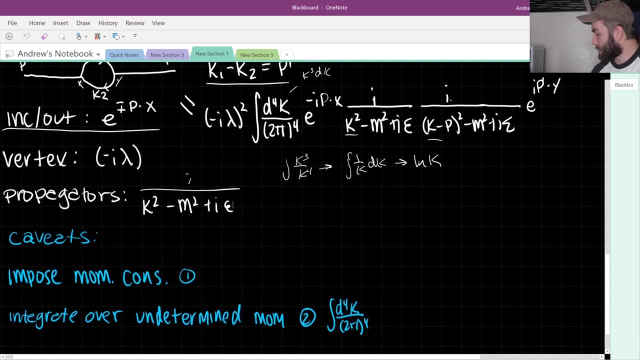 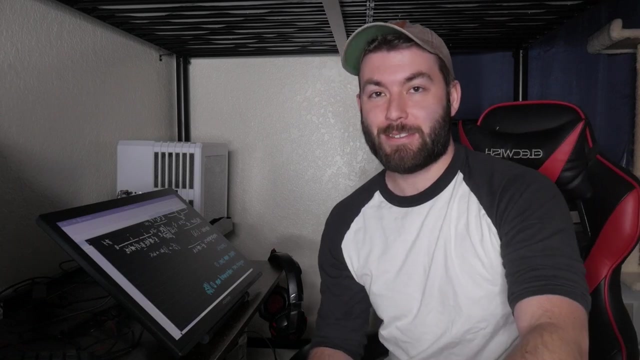 actually less favorable, which which is definitely the case, especially in some, like, weak interactions. but that's what I meant by by complicated diagrams contributing less, and that's that's really all there is to it. that is how. that's, that's all there is to it. all that's left is to actually evaluate those integrals. but these are 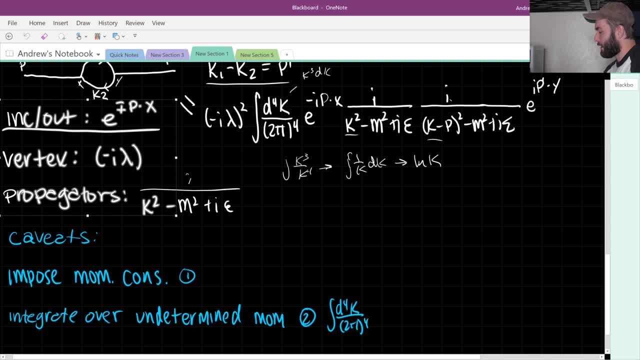 the parts that make up the Feynman diagram- the incoming, the external legs, vertices and propagators- and to translate them into math. you just have to look up the Feynman rules for whatever theory you're considering. now I'd like to take just a couple minutes of your time to talk about the tablet. 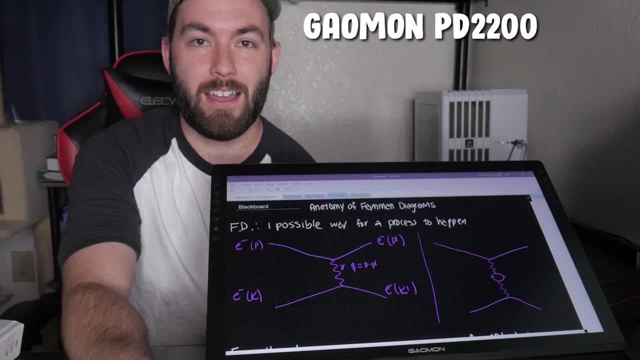 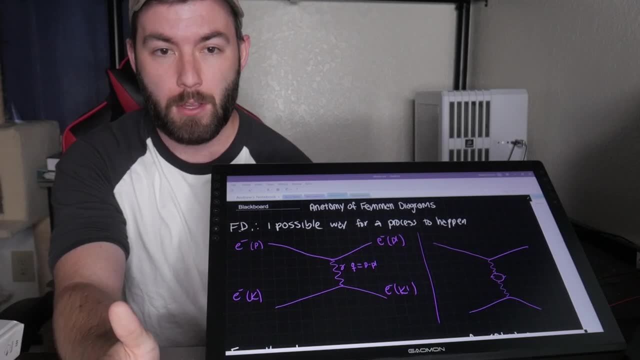 that made this video possible that I was just broke just now: the Gaomon PD 2200. I made a video previously with the PD 1560 that they sent me, which is phenomenal now that I have two, I ended up giving that one to Kelly and she uses it every single day. awesome tablet. the 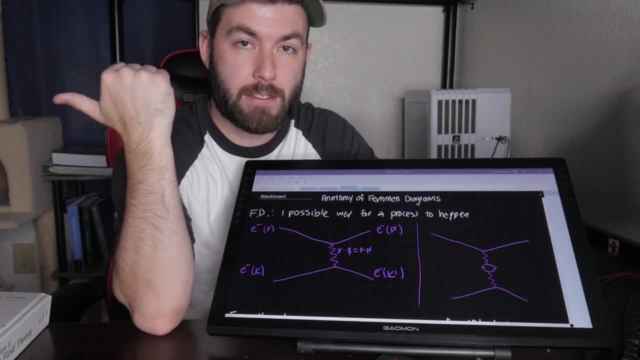 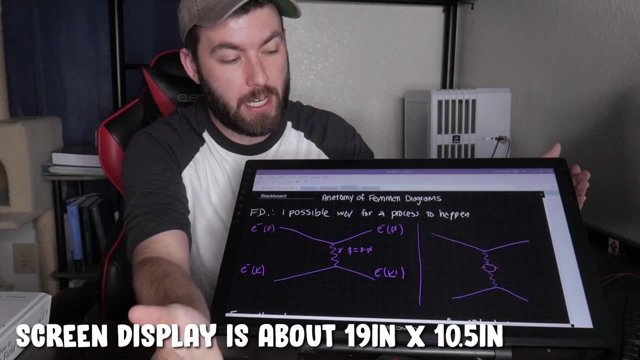 primary differences between this and the PD 1560 from the previous video. well, for one you can tell this is a much larger screen, a lot more surface area that you can work with, so I don't really run into issues of running out of space or having 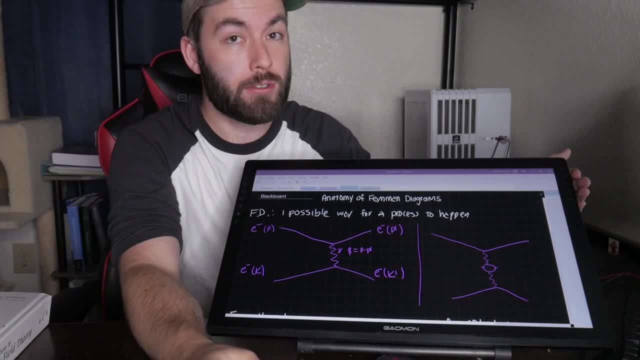 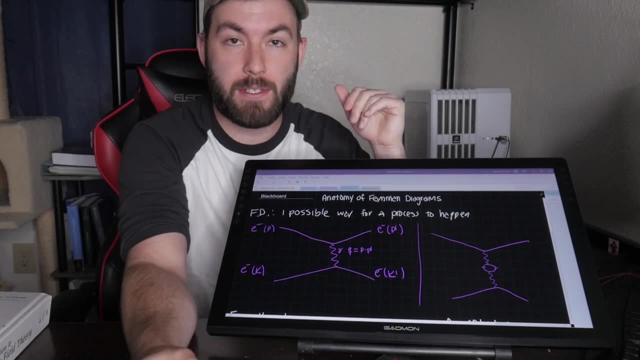 to move to different lines, to write out the single equation, which you should be surprised how often that happens. so that's like the biggest thing for me is I have more space to work with. there's also more customization options as far as presets that you can set go, there are eight. 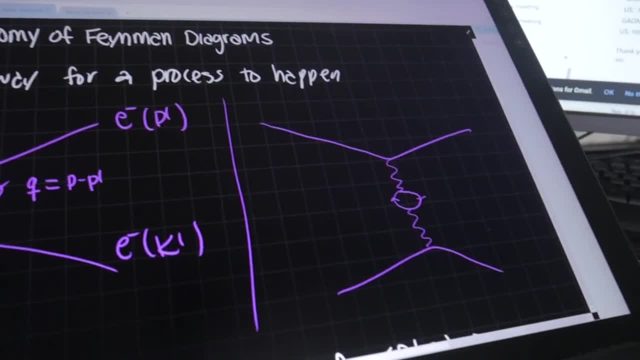 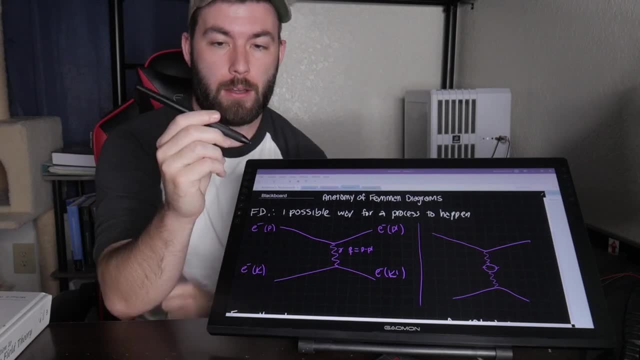 buttons that you can select on the side of the screen, as well as two on the pen itself. now, I'm a simple guy so I only use like three of them. I like to have an eraser. I like one button on the pen for pen selection. the common pens that I 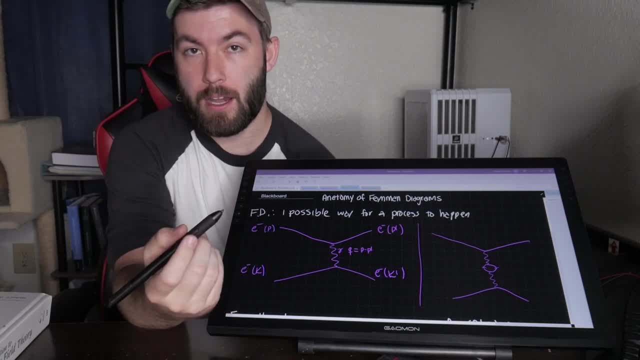 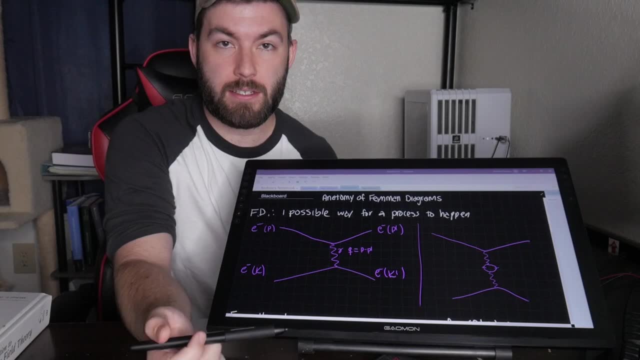 like to use, like the colors, and then one for click and drag, and then I'm happy with that. I also have a pen holder for my keyboard, if you want to use a pen holder, if you need additional options. now, this is not, it's a touchscreen in. 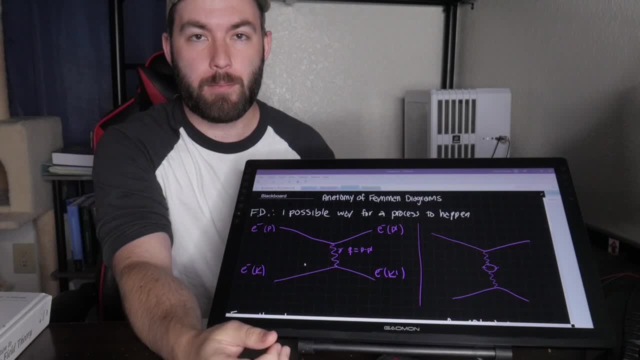 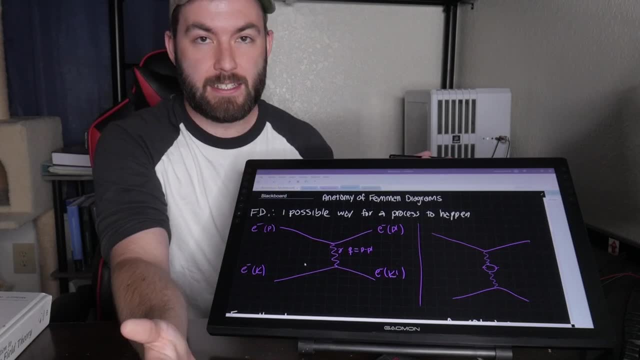 the sense that you can use your pen on it, but it will not move if you're touching it with your hand, which I guess is both a good and a bad thing. this is the same for pretty much all of these style of tablets, by the way, it's not? 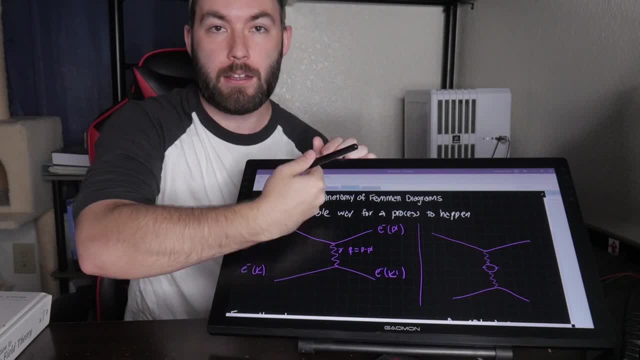 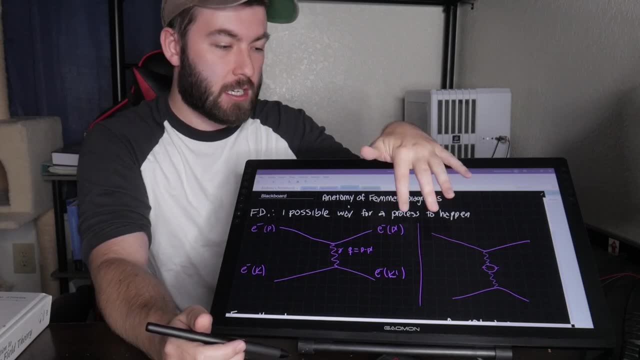 just Gaomon. the reason I say it's not necessarily a bad thing is because you don't have to worry about dragging anything over when you're writing on the screen. that's why I could have my hand on the screen and it's not shifting things around. but you can't just touch things with your finger and select things. 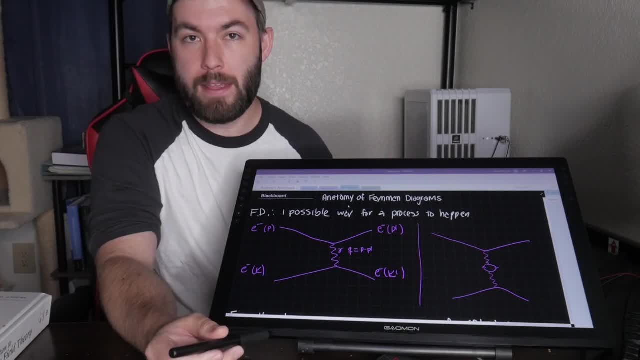 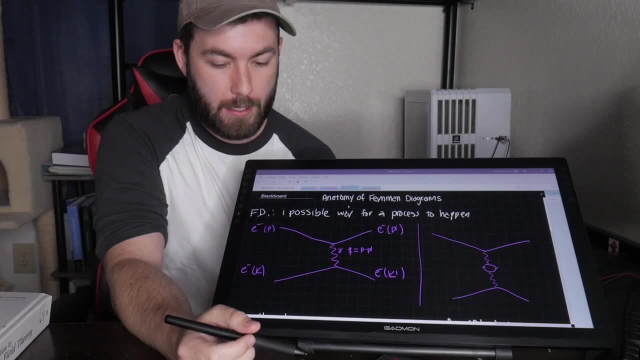 which is one thing to consider. that hasn't been a real issue with me, because you do the same thing with your pen anyway with selecting it, so that hasn't been a problem with the 1560. the one thing that I wasn't a huge fan of was: 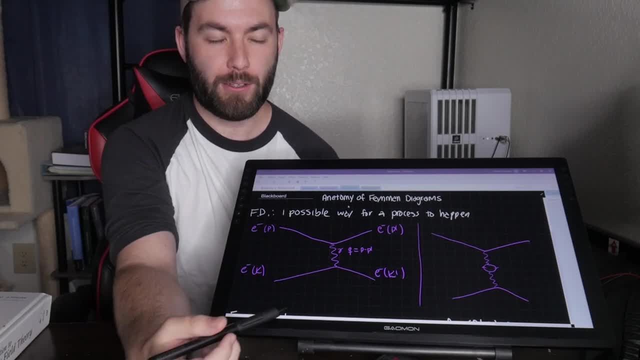 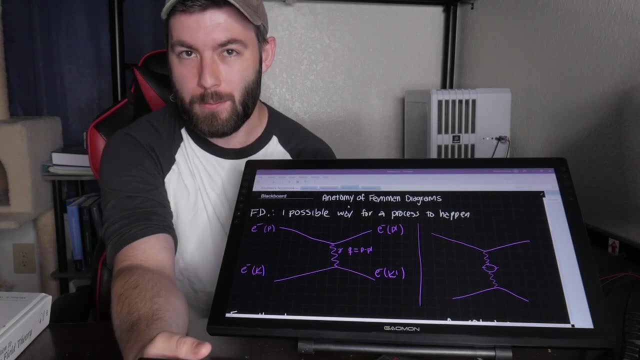 the friction II feel with the pen on the screen. it felt like I would eventually scratch it, even though Kelly and I have put that thing through the paces and there's not a scratch on it. it just felt that way for some reason. this is a much. 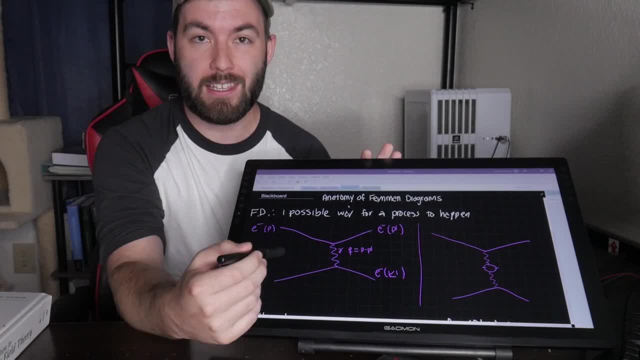 smoother surface and it's not a scratch on it. it's not a scratch on it, it's not so. I don't feel that at all, and the pen that it comes with gives a little bit, giving it a softer feel, which is nice. I don't have too much else to say about it. 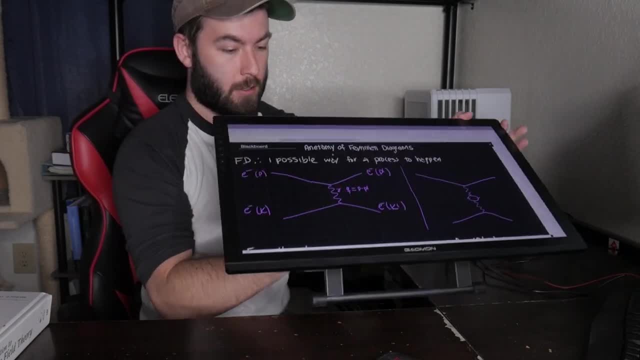 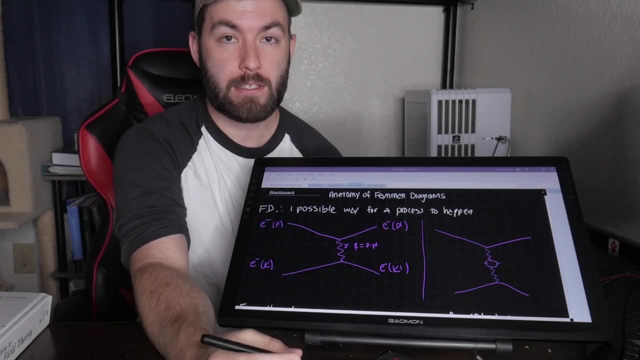 there's also a stand that is adjustable so that you can get a comfortable angle, so it's not just flat on the ground. it has to be plugged into a computer. so if you're someone who works in the same spot every day or if you do all of your, 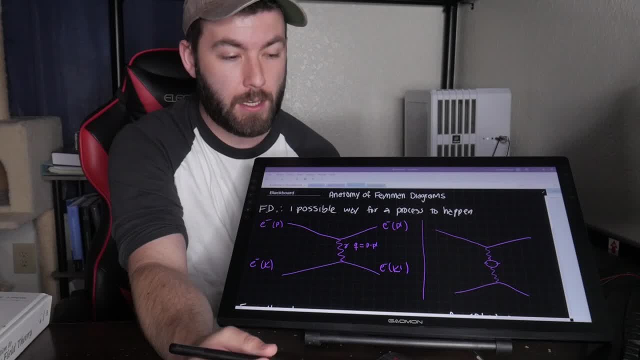 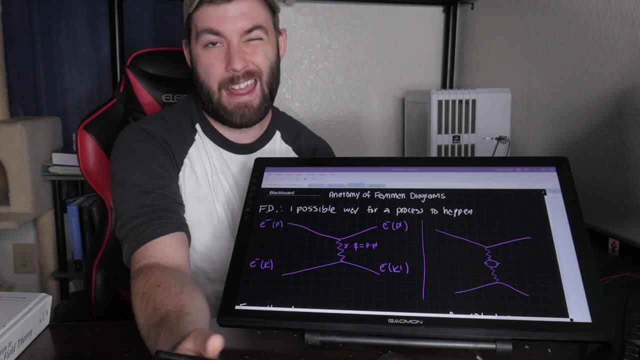 work in one spot. this is definitely a fantastic option if you're someone who needs to grab things and go. I mean, you can do that as well so long as you have a laptop, but it's just not as portable as I would like it to be, but it's also. 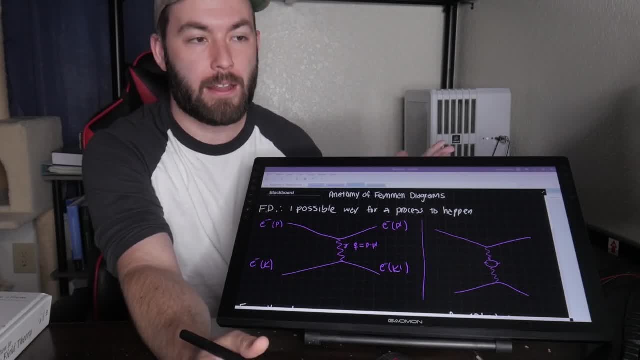 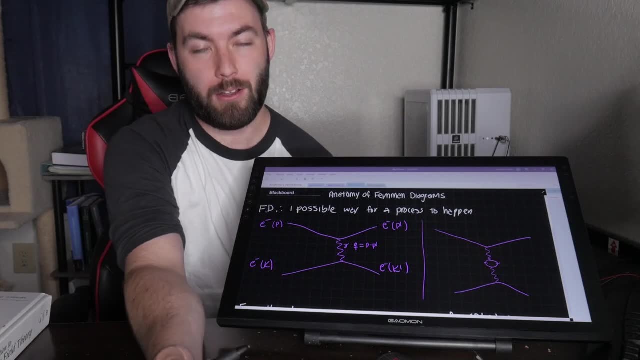 massive. I don't know why you would carry this thing. you know this isn't for that. this is for staying in one spot, really, and getting the job done. so if you want to find out more of a comprehensive review, I'll leave a link to flammable 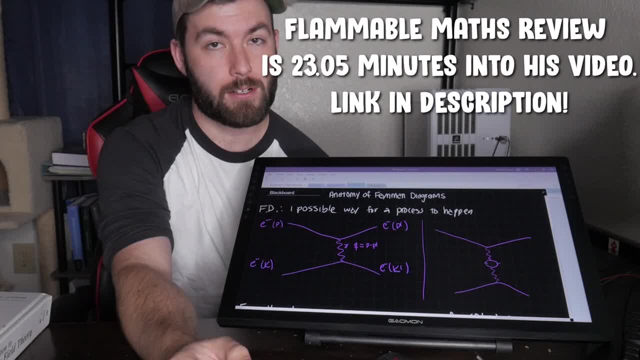 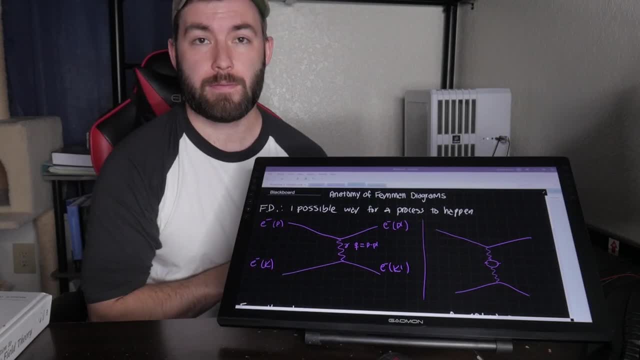 mats video, and you can go to this section of the video, to where he starts reviewing the tablet also leave other links to videos that are more dedicated. so thanks to Gaumont for sponsoring this video. you can click the link in the description for future videos and I'll see you in the next one. 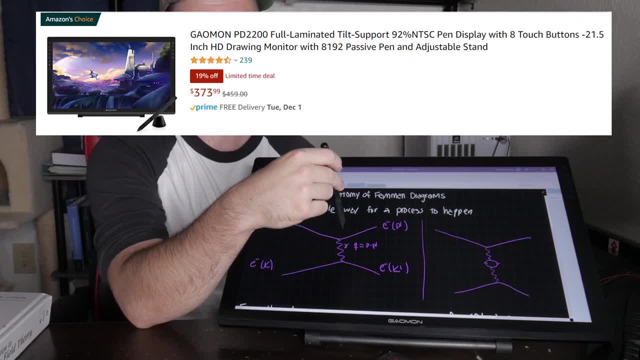 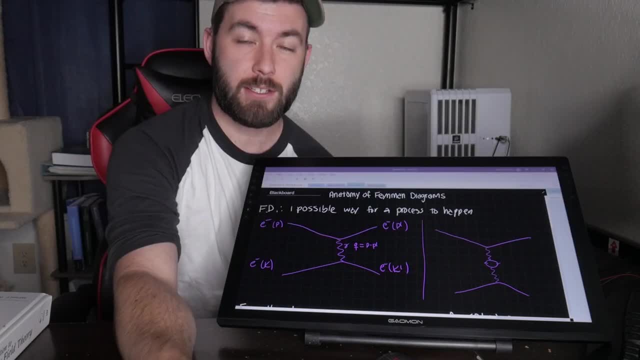 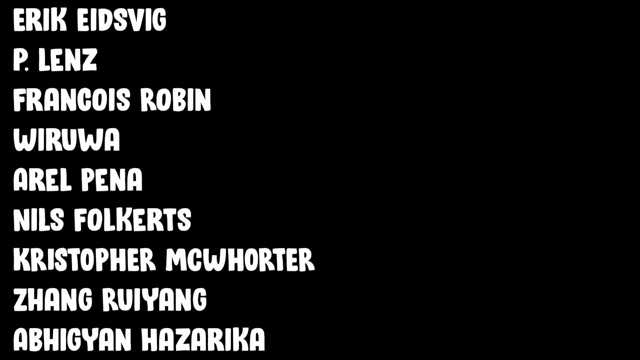 15% off of this tablet, the PD 50, PD 2200 or 34% off of the PD 1560 for the Black Friday sale. thanks to sponsoring this. hope you guys enjoyed this video. let me know in the comment section if you did and I'll see you guys there.